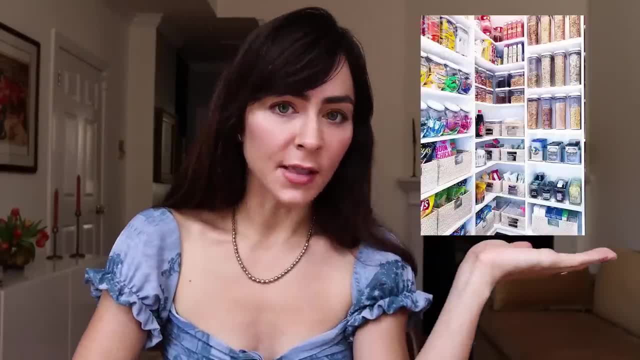 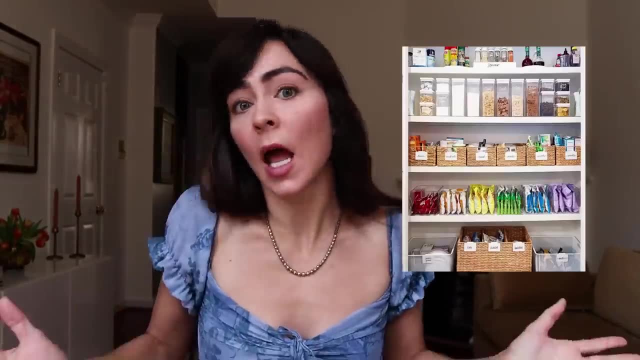 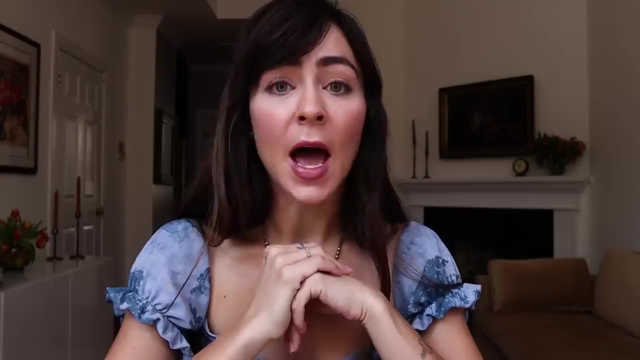 Okay, don't get me wrong. I find this brand of medical grade pantry organization to be just as sexually satisfying as the next guy. Okay, I get it, I like it. However, this brand of home organization is never going to give you an organized home. Not only is it expensive, but it. 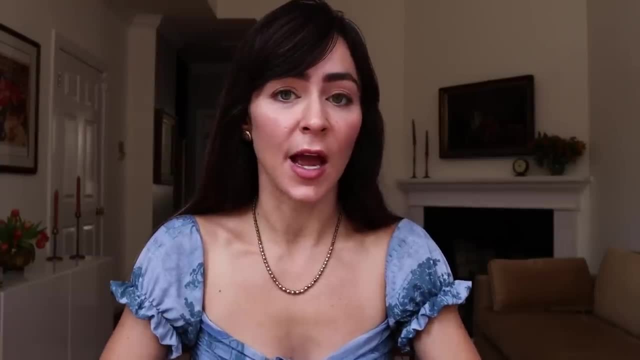 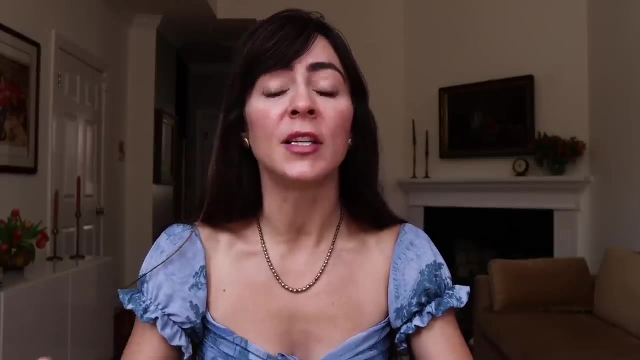 usually doesn't even fix the real problem. When I have an interior design client who has a messy home, the problem isn't usually that their M&Ms aren't color-coded. The problem is that we all have a ton of stuff and we don't know how to get rid of it. We don't know what to get rid of. 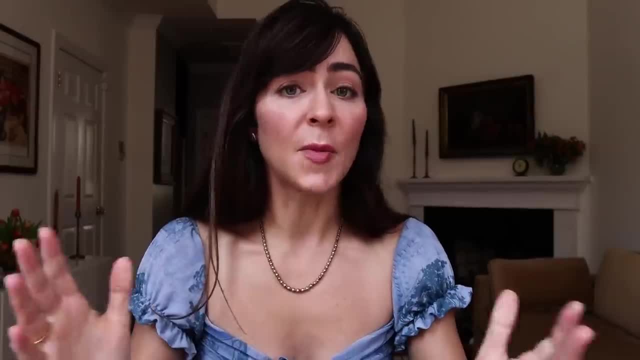 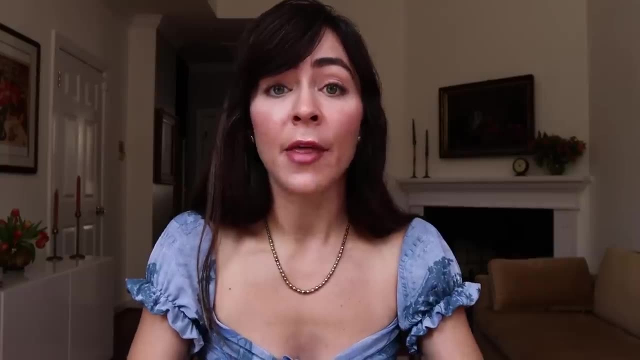 and we don't know how to arrange the things we actually keep. And you can spend all the time in the world pinning images on Pinterest and trying to design the perfect space, but if your floor is covered in clutter, then it truly doesn't make a bit of difference what rug you end up buying. 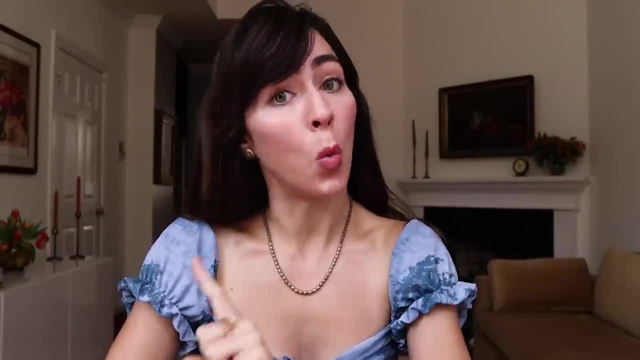 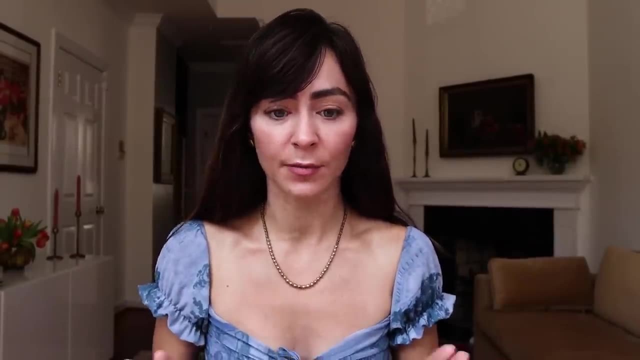 I'm going to tell you which organization products are worth getting, which are not and, more importantly, the organization design principles that will keep your home organized and running smoothly. My name is Caroline And this is home organization from an interior design perspective. 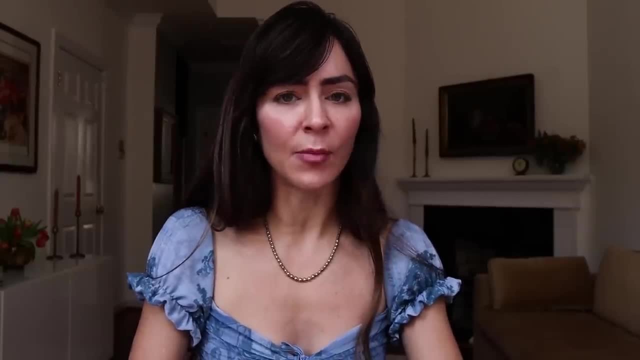 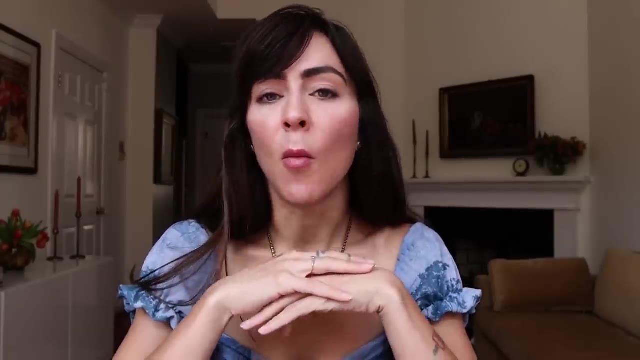 Every home organization video on YouTube is pretty much telling you the same thing: Buy this, buy this, buy this hack, buy this gadget, buy this product, consume. Home organization is about more than just products and gadgets and hacks. It's about systems that make your life. 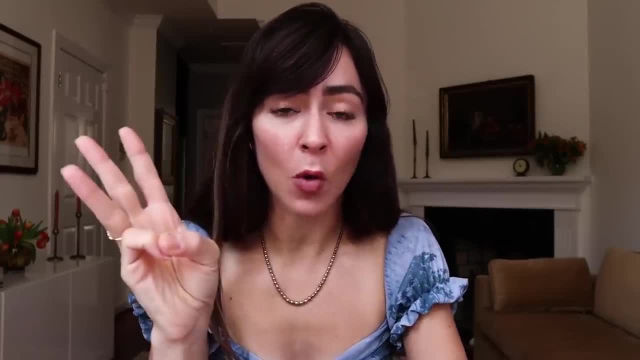 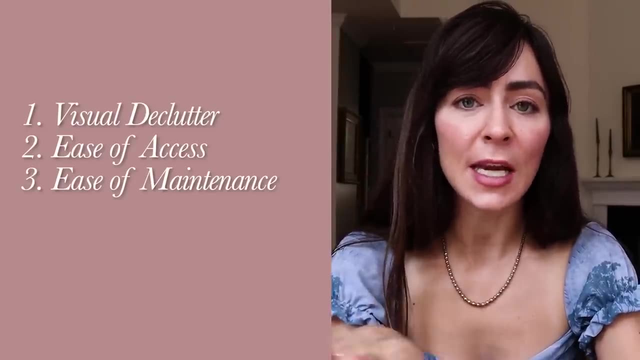 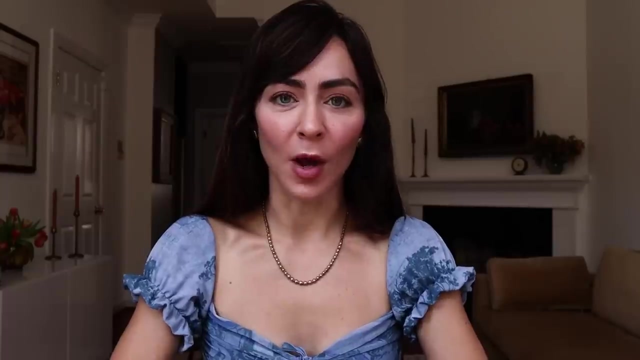 work better And great home organization has to meet three requirements: Visual declutter, ease of access and ease of maintenance. And we're going to get into all three with 10 tips to keep your home organized. Tip number one: corral your crap. This blows people's mind If you're looking at your nightstand. or your kitchen counter. you're going to see a lot of people saying, oh, I don't know, I don't know, I don't know, Hey, I'm going to go to the coffee shop or the coffee table And you're like ugh. 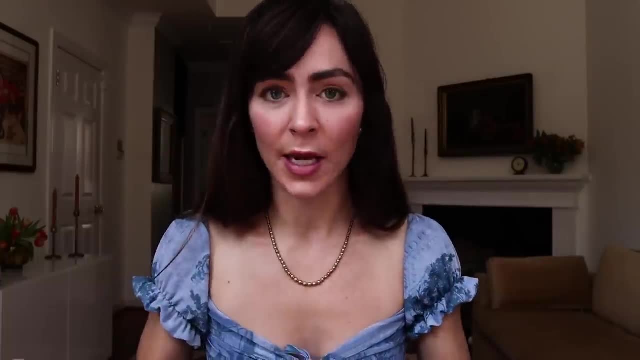 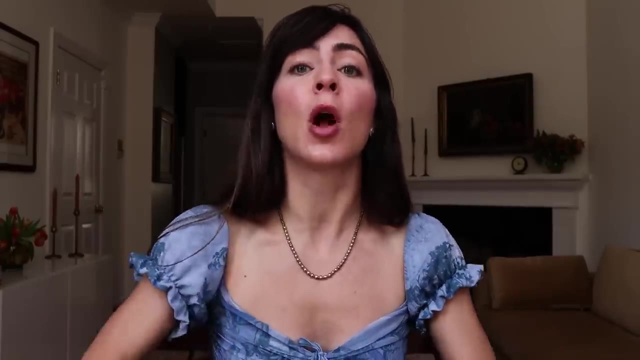 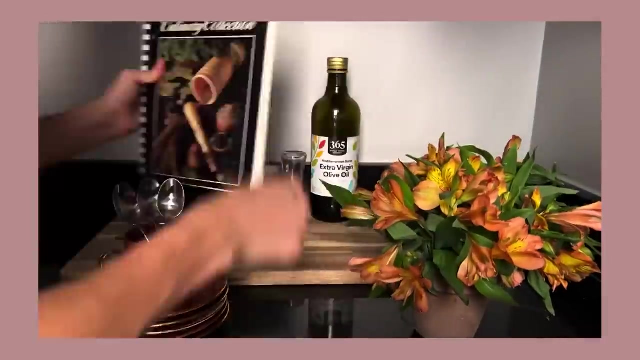 it's just a lot of stuff. It's visually busy. Corral it Just place things on a tray. It will blow your mind at how quickly it solves the problem of visual declutter. And it doesn't have to be a tray: You can use a book, you can use a cutting board, You can use a stack of magazines. 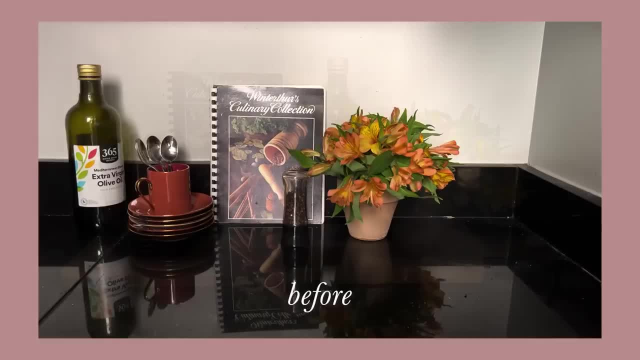 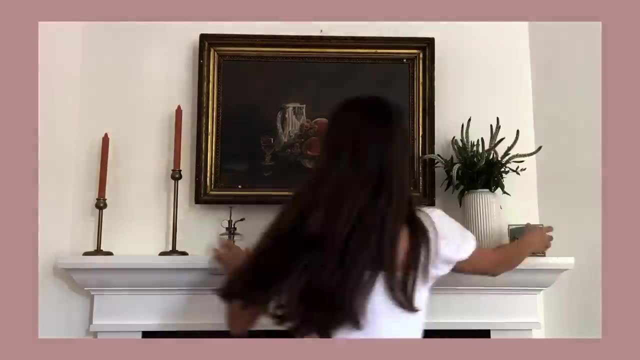 something that takes a bunch of individual items And then instead of five items you just have one item- It sounds like semantics, but it makes a huge difference- And group items in groups of threes. even without a tray. this can make a huge impact, varying the 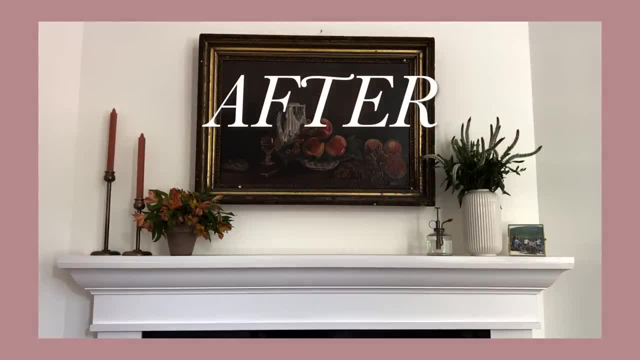 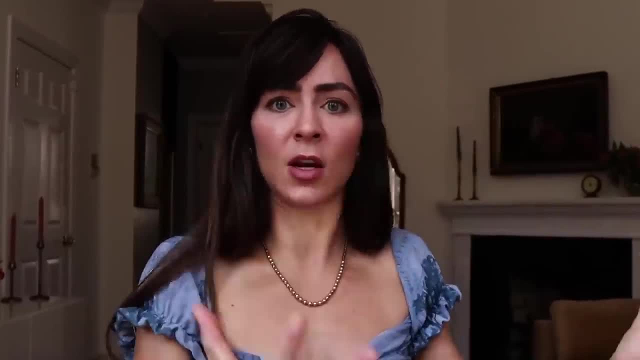 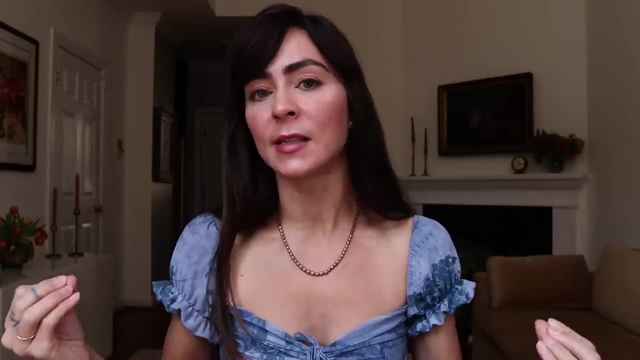 height of those items. so they they kind of become it's kind of like transformers or the Power Rangers or what's the ones- that they all come together and they make a new thing. yeah, you group things together in groups of threes, they become a new item, a single item, and it minimizes the visual busyness. corral. 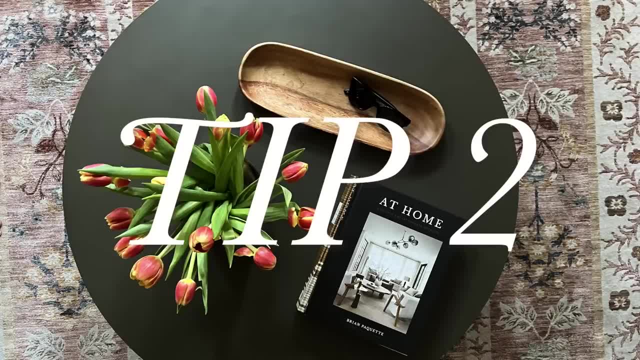 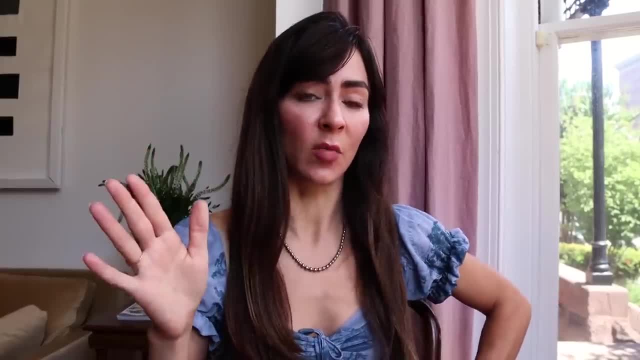 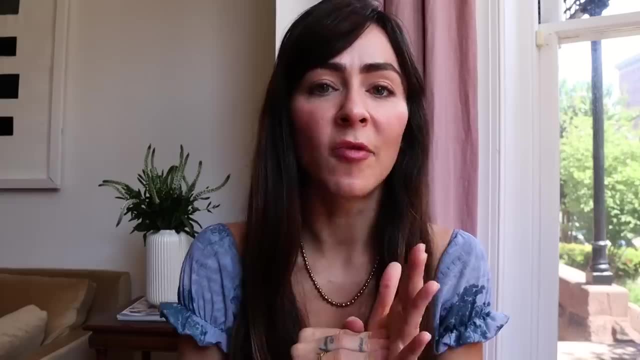 that's it. that's it. tip number two is another gadget that I fully endorse. in fact, I insist upon it: velvet hangers for your closet. don't talk to me about other kind of hangers. these are the only hangers I use. clothes never fall off the. 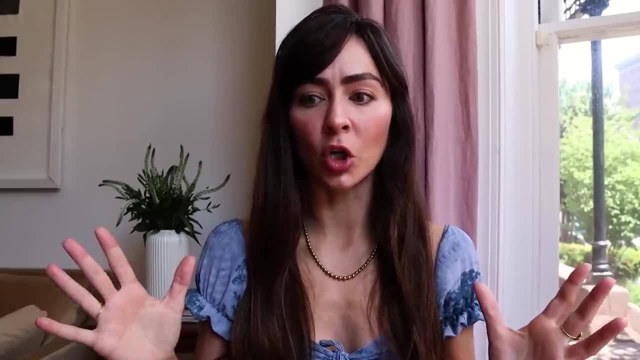 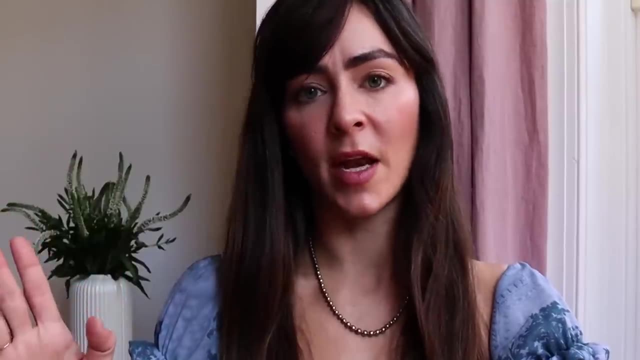 velvet hanger. normal hangers, non velvet hangers- are just another form of misogyny, trying to punish women for owning camisoles. don't let them stop you. buy the velvet hangers. it's a great way to get rid of your hangers if you're. 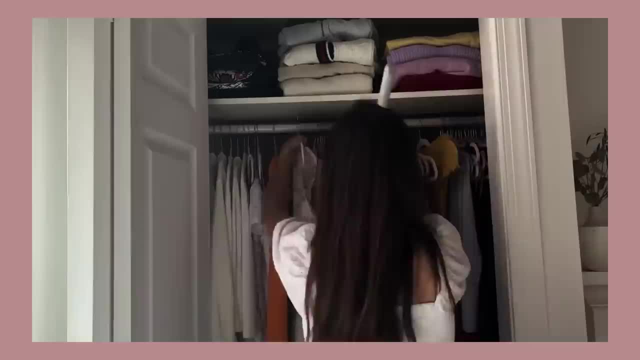 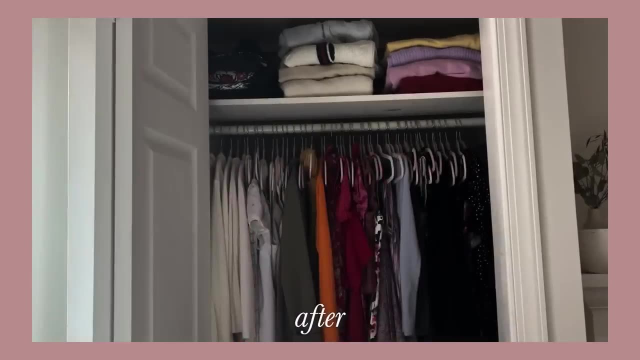 going to keep them forever. it's an investment. you invest once, you keep them forever. and yes, it's nice to just get all one kind of hanger in your closet. that's already like the visual declutter satisfying. you'll feel a little bit high, but the difference is that if I fill a closet with wire, 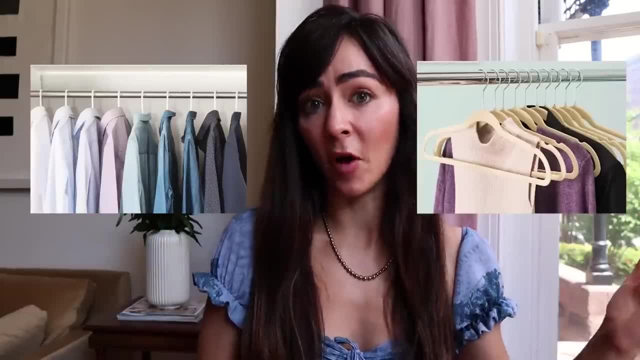 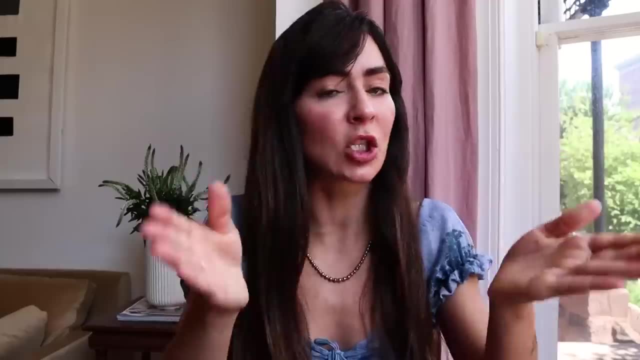 hangers or plastic hook hangers and I fill a closet with velvet hangers. only the velvet hanger closet is gonna stay that way. okay, I don't. I don't have the seconds to put the spaghetti straps into the little hooks and the clip in the 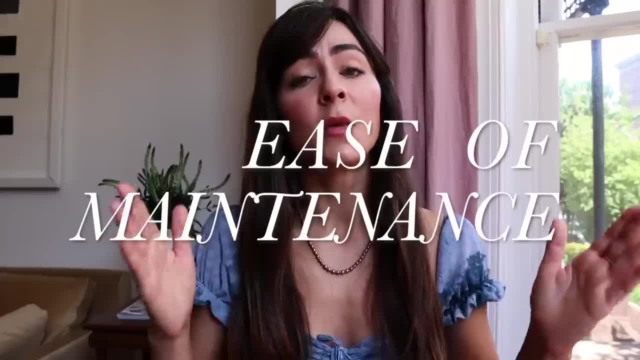 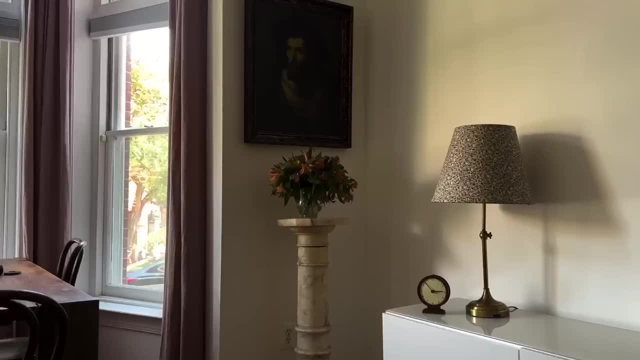 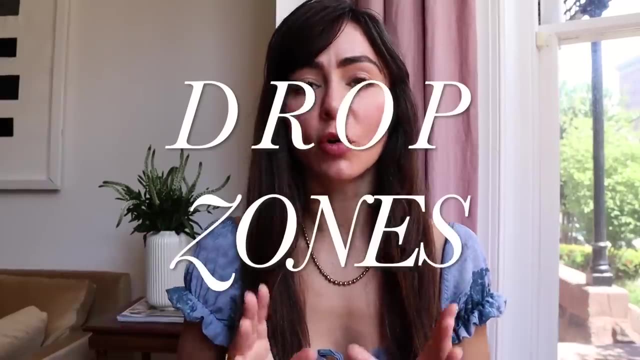 I have a life to live. I'm a busy lady. make it as easy as possible to get those clothes put away, and they'll stay put away. end of discussion. end of discussion. this is a big one: drop zones, creating intentional drop zones where the key's going, where's the coat going? 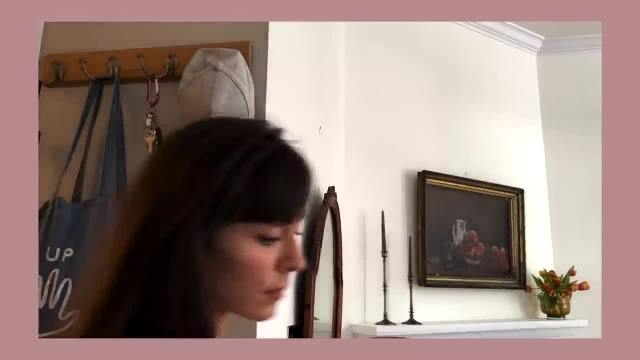 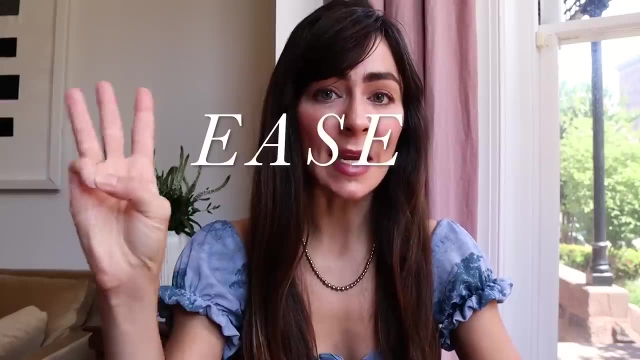 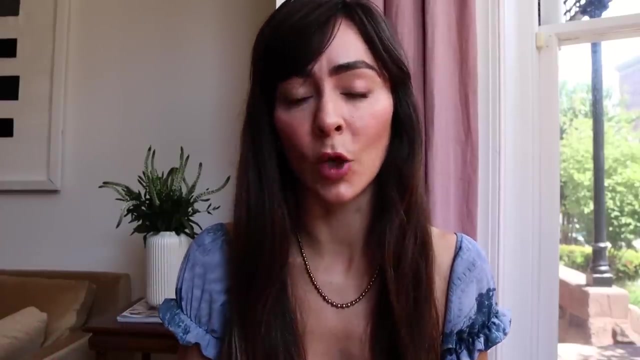 where's the bag going? it sounds simple enough, but the way you create these drop zones is extremely important. and that gets us into home organization. requirement number three: ease of maintenance. And this one is the most important, because if it's not easily maintained by everyone in the home, then it's not going to work. There's nothing more impossible than. 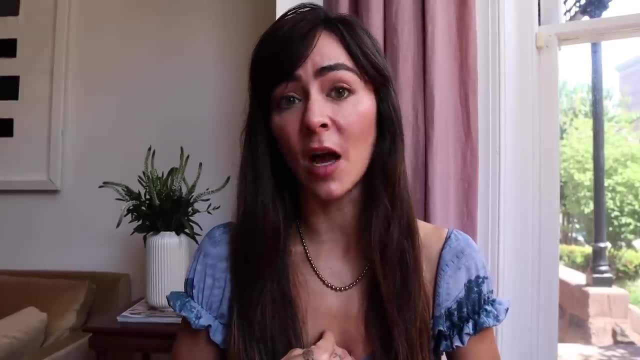 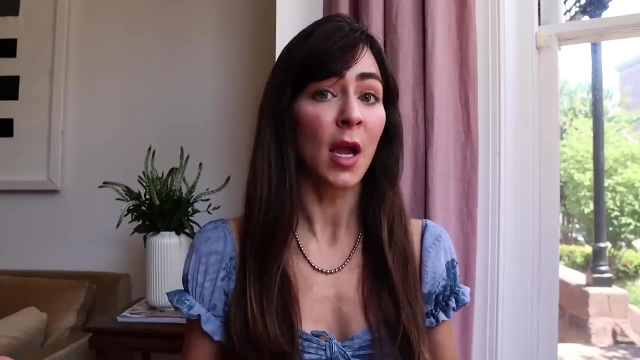 changing human behavior. It's hard to create new habits for yourself, let alone for me to create new habits for my pretend partner or my pretend kids. And if they can't uphold my new organization system, then I'm left doing it all alone. And that's not why I got pretend married The best. 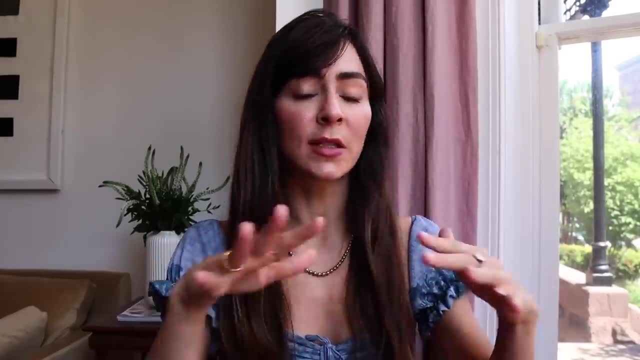 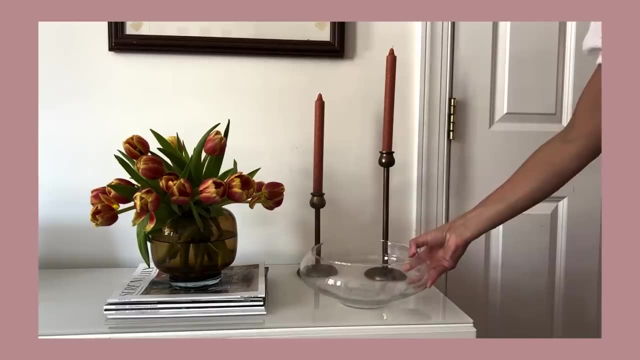 way to create drop zones is to watch how you, your roommates, your family watch where you are naturally dropping your stuff when you come home and then put the drop zones there and just make it intentional. If all the keys are always going on the table, put a freaking bowl on that table. 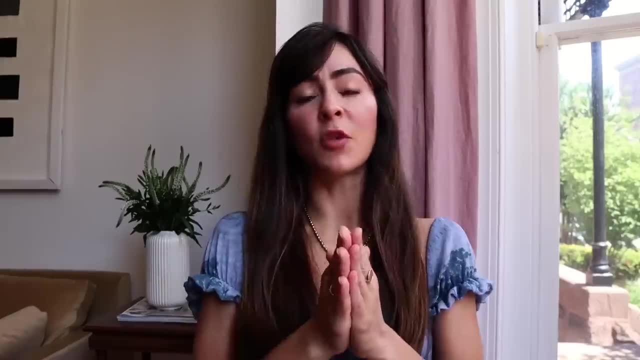 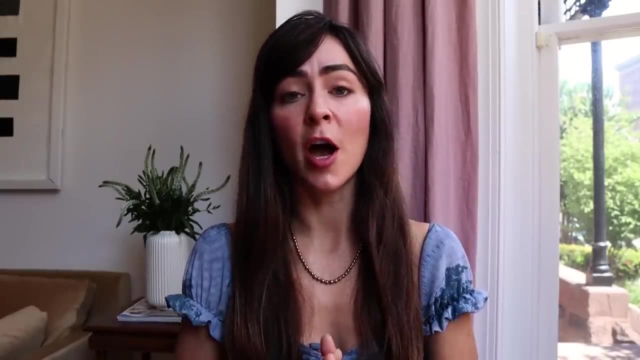 If the coats are always going in that corner, put a hook in the corner. If the bag is always being dropped there, put a table, put a chair, put a stool. Good design and good organization systems are not about making people adhere to your system. 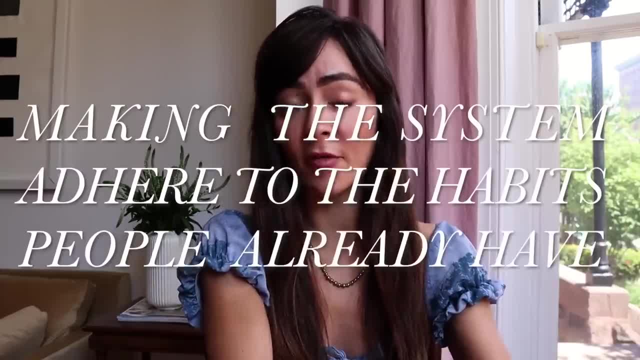 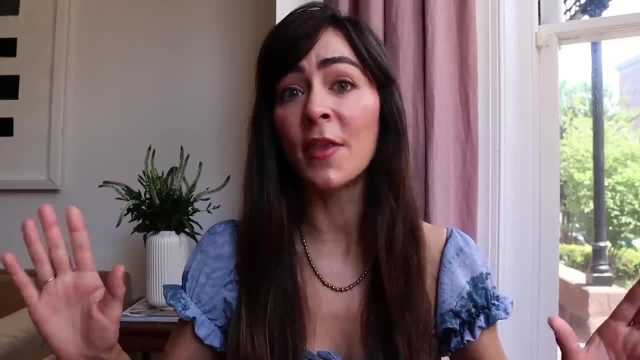 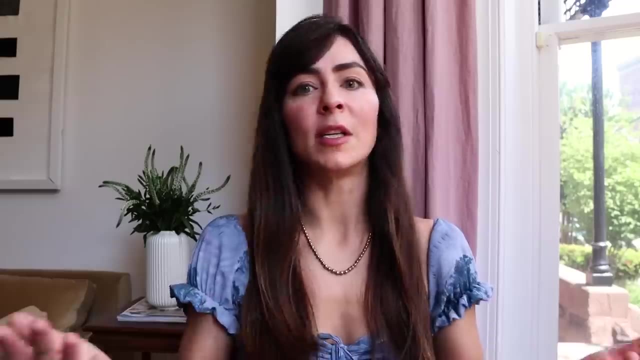 It's about making the system adhere to the habits people already have. It's about making the system adhere to the habits people already have. That's the way they get maintained. So if we don't consider ease of maintenance, then the drop zone could easily be on the other side of the room. What does it take you? four? 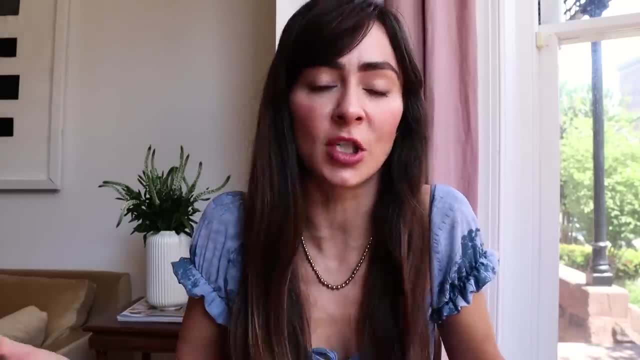 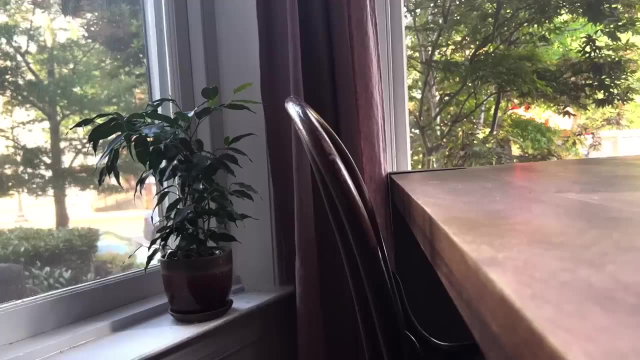 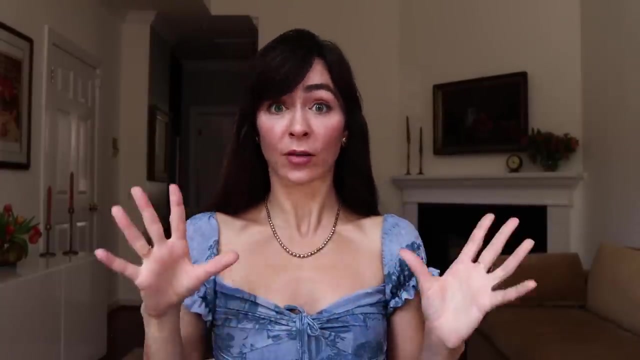 steps to get there and put your coat down. Easy access: It's not hard to access that, but it's hard to maintain it. If it's just a little inconvenient, it's not going to happen. Tip number four is one of the very few home organization products that you I highly 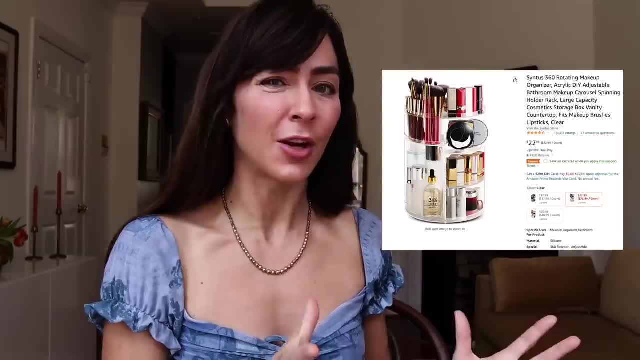 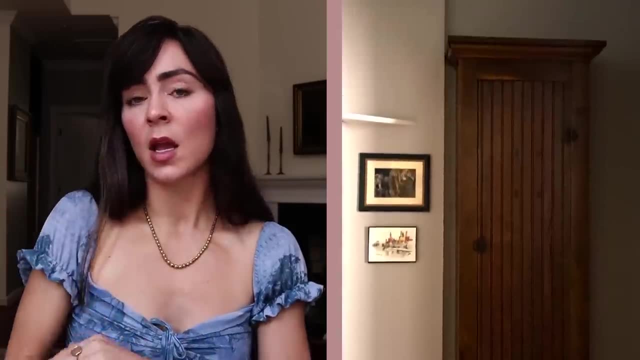 recommend. You should definitely get this. There's a bunch of versions of this tiered Lazy Susan that you can get online. I got mine off Amazon. I'm using two of these in my tiny little linen cabinet. It holds all my toiletries, all my medical stuff, all my travel products. 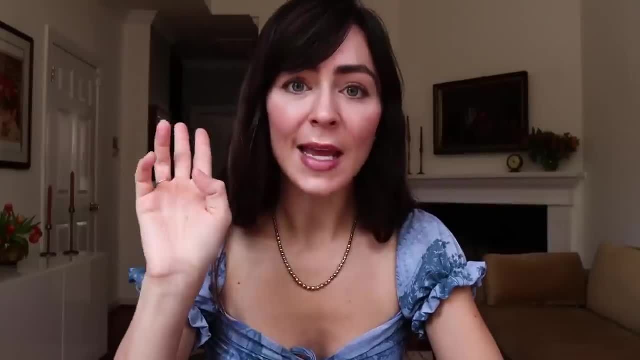 This product gets us into organization. principle number two: ease of access. So, yes, we want to visually declutter and we want to make sure that we're not getting in the way of the organization, And we want to make sure that we're not getting in the way of the organization And we want to make 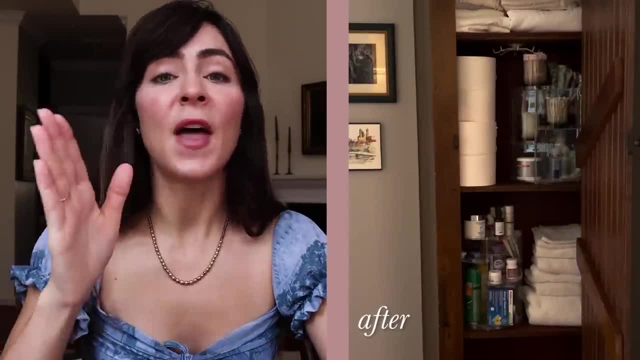 sure that we're not getting in the way of the organization And we want to make sure that we're find a place for everything. We want everything to have a place, but if that item cannot be easily accessed when you need it, then it's never going to go back there. It's never going to go back to. 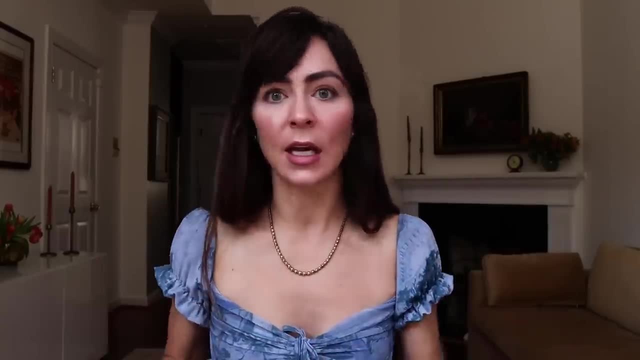 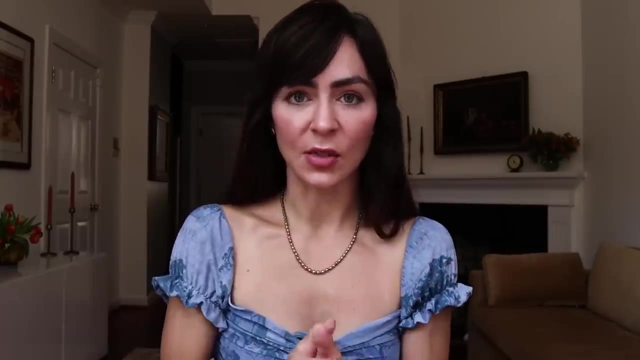 that place. This is why just getting a box for everything, just getting an expensive container store container for everything, doesn't solve the problem. It's how you organize it. Before I bought these Lazy Susans, I had to pull out five drawers and a bunch of stacked shelves and I couldn't get. 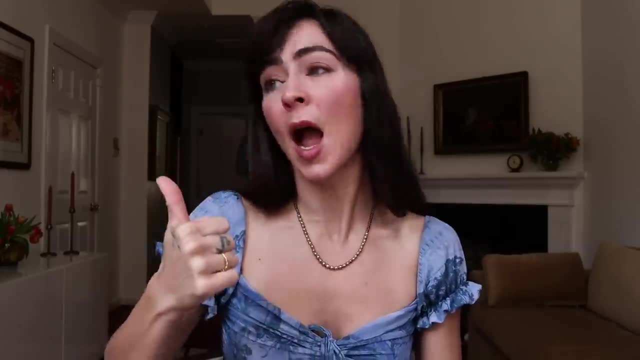 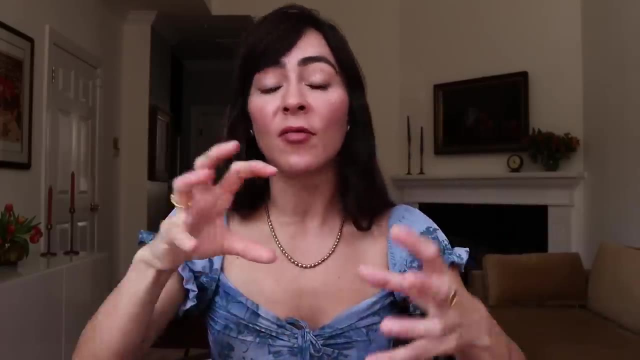 to the things, And then not only by the time I'm going to get my tube of toothpaste, I'm furious. First of all, I'm pissed off, And it's probably not going to get back in that place either If it's too hard and I have to pull everything apart to get it out, This tiered Lazy Susan. 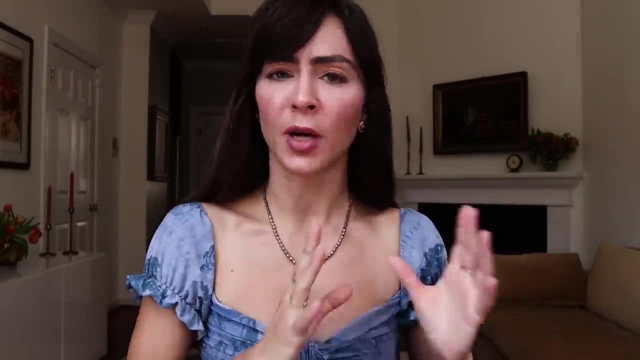 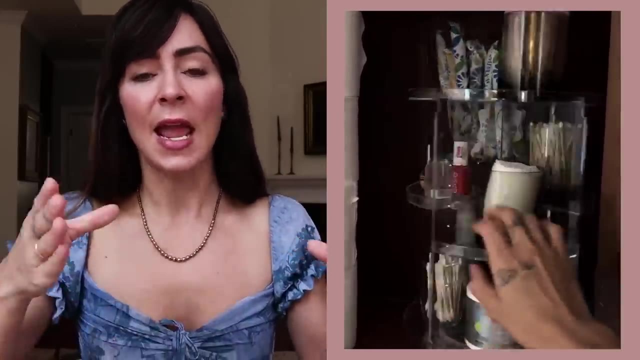 makes so many things, so many items accessible. There's a bunch of versions of this, but this is the best version in my humble opinion, because there's no wasted space. You can adjust the shelves, and the shelves don't get too compartmentalized. It's one thing you have to. 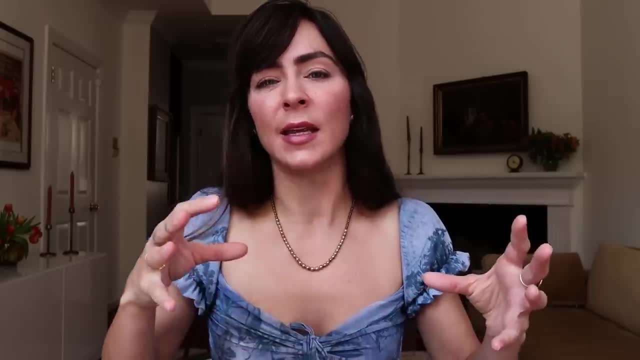 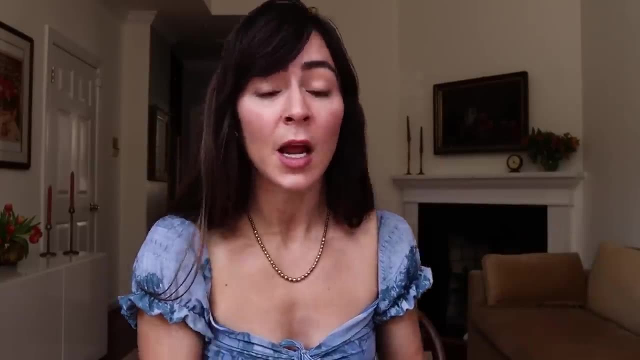 look out for Sometimes they get too divided and it limits what products you can put in there. It's pretty enough that you can display your makeup on it. You can display your perfumes on it. I personally, I like to just leave my perfumes out on the vanity or in the bathroom because they're 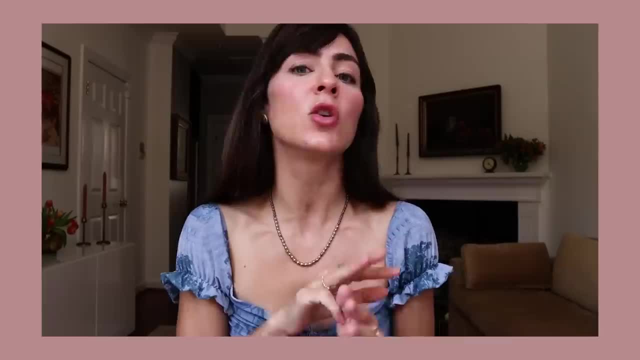 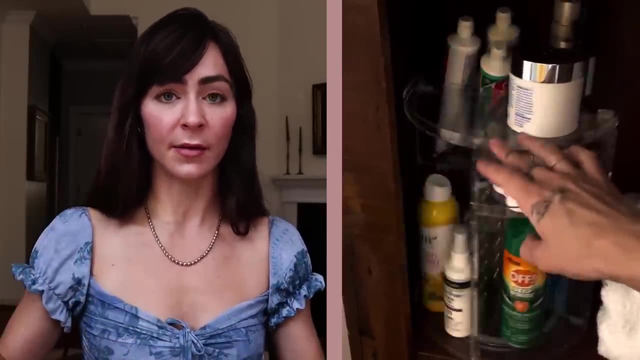 kind of. they're little statues, They're little pieces of art themselves, So I don't really like to squirrel those away. This tiered, Lazy Susan makes so many items accessible without you having to touch anything. Do it. I recommend, If you're like me and you're trying to save money, so that 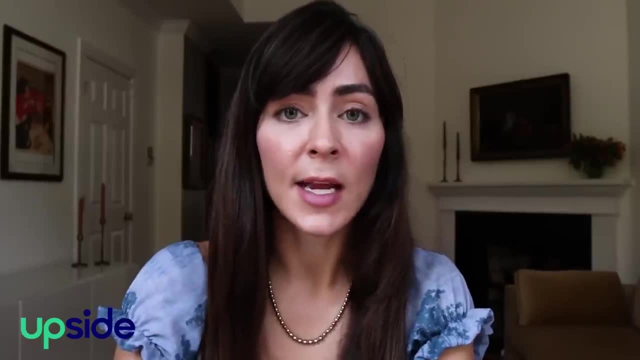 you can blow it all on home decor Upside is one of the easiest ways to save money. It's a cashback App that basically sounds too good to be true, but it's not. I'm a pretty skeptical person. I've used the app myself and I'm here to spread the good news. Bless me. Anytime you make gas grocery dining purchases, you get cash back. It's super straightforward And that's probably why they have a 4.8 star rating on the Apple store. Recently I found myself cringing at gas prices. 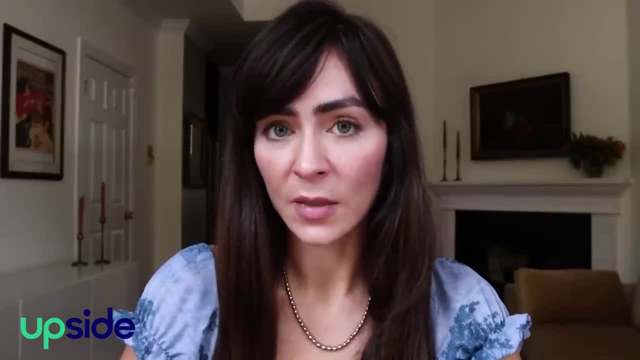 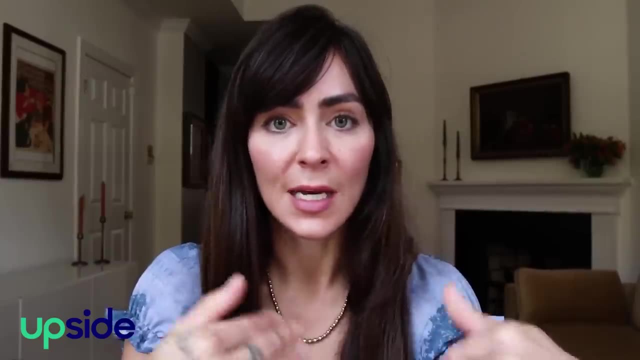 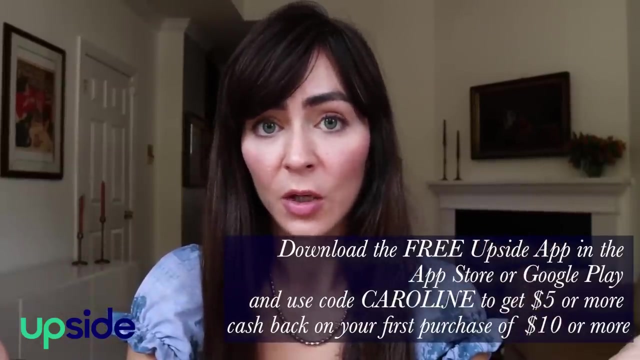 You may relate, and God forbid those gas prices. keep me from buying yet another vintage vase off of Etsy, God forbid. To get started, you just download the free Upside app and use code Caroline. It's me To immediately get $5 back on your first purchase of $10 or more. 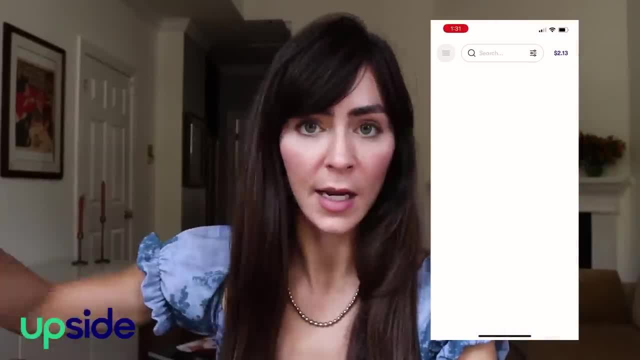 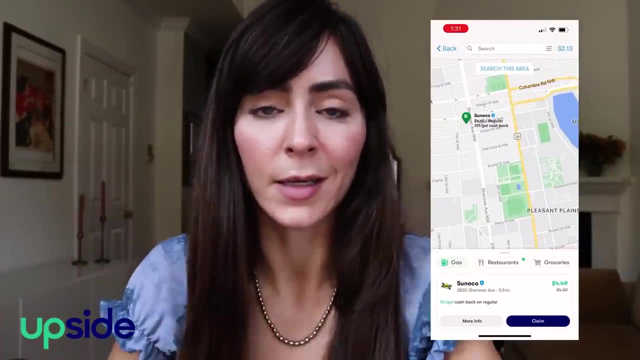 Then next you show up at the place that you're doing- groceries, dining, gas, whatever- You check in at the business. on the app, You pay as usual with a credit or debit card and you get paid. It is super simple, Instead of losing my entire life savings at the gas pump. 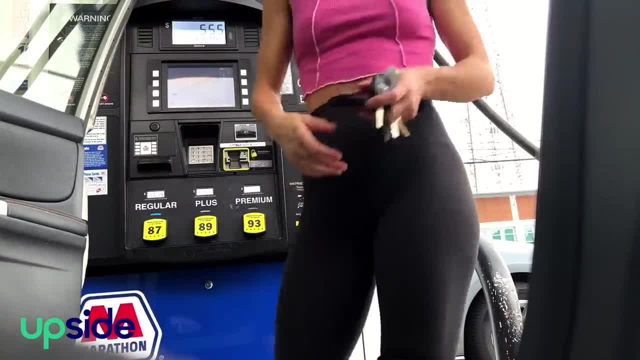 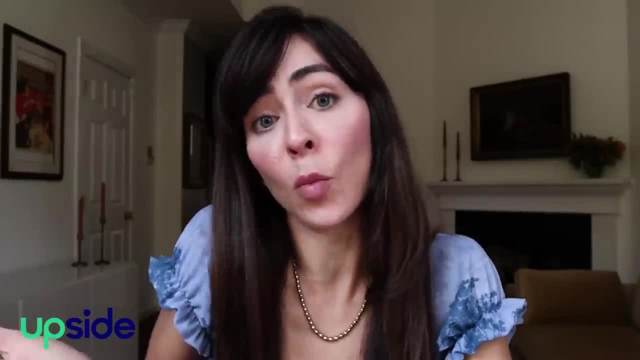 I've now started using the Upside app and you can cash out at any time, To your bank, to PayPal, to Amazon gift card, whatever It's very convenient. I'm going to be buying gas, I'm going to be buying groceries. It's a no-brainer to me. to go check in on the app and get cash back. The very first time I used it I checked in at a gas pump. I got cash back in my account the next day. It's super simple, super easy to use. Highly recommend checking it out. It's a no-brainer. 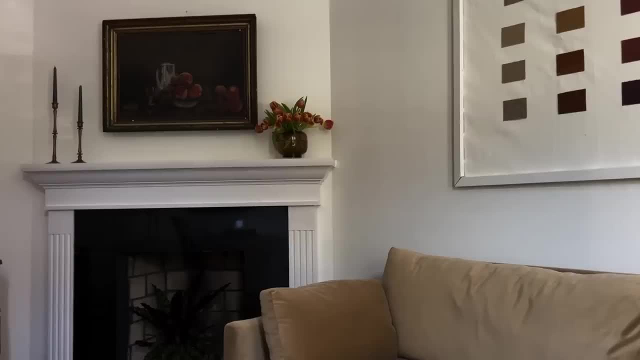 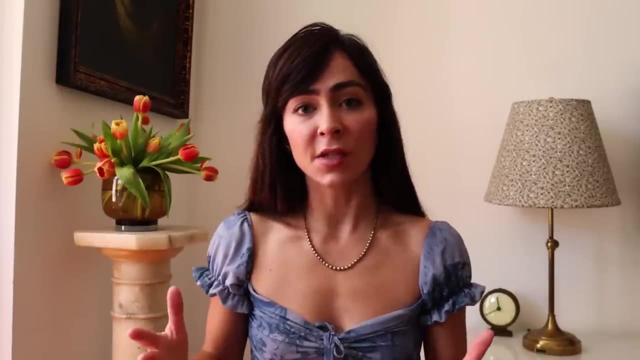 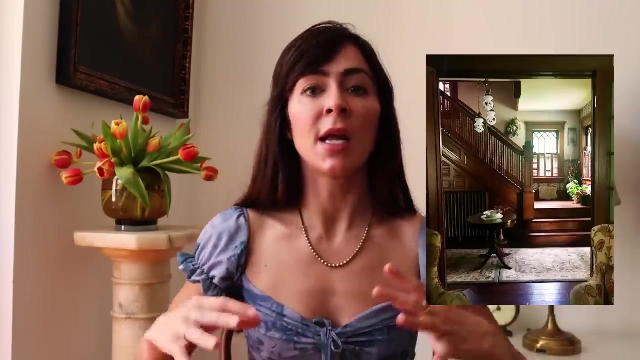 And thanks to Upside for sponsoring today's video Tip number five: active zones versus passive zones. We got to define them. Active zones are the areas in your home where you're moving stuff all around. You've got your entryway, maybe your living room, kitchen Stuff's coming in and out. We're dropping stuff. 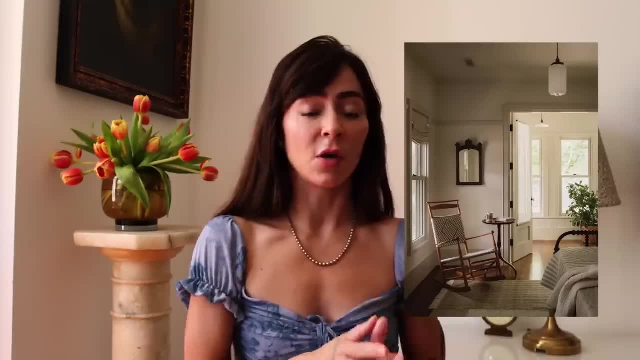 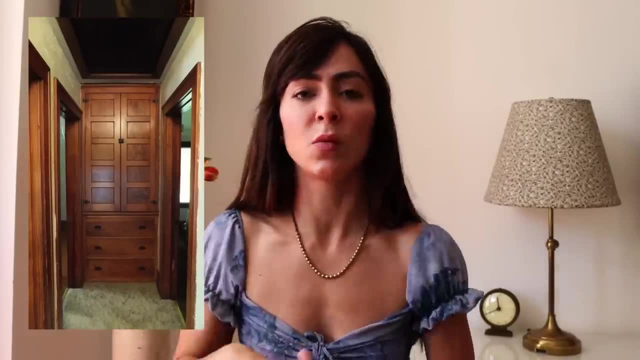 We're taking stuff, We're really living in those spaces. Passive zones are maybe your guest bedroom, maybe parts of your basement, maybe that back closet that we never really access. Whatever that is for you. we got to define those areas because not all storage areas are created. 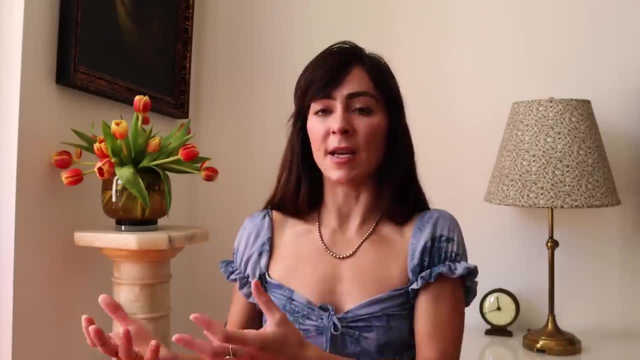 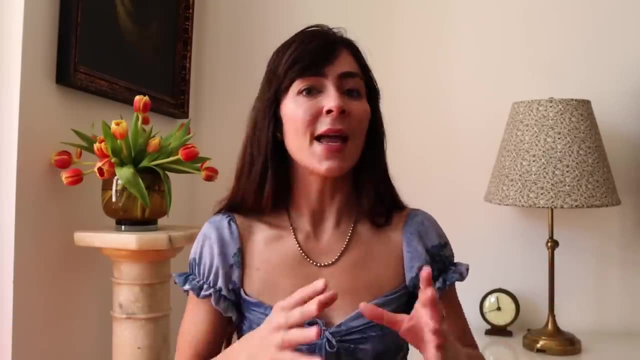 equal. A lot of people make the mistake of putting items that they only need to access once a month or so in an active zone. Don't put your spare light bulbs that you only need to change out once every few months in an active zone. It's just taking up space. Put it in a passive zone. 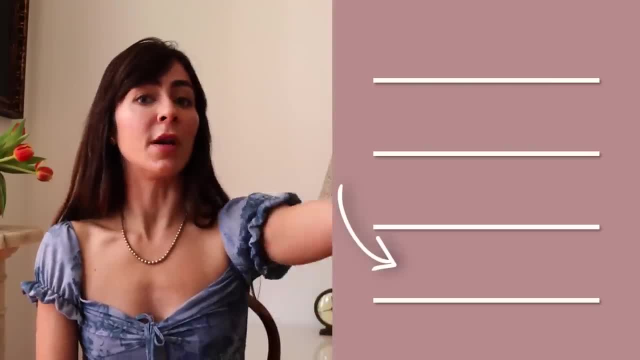 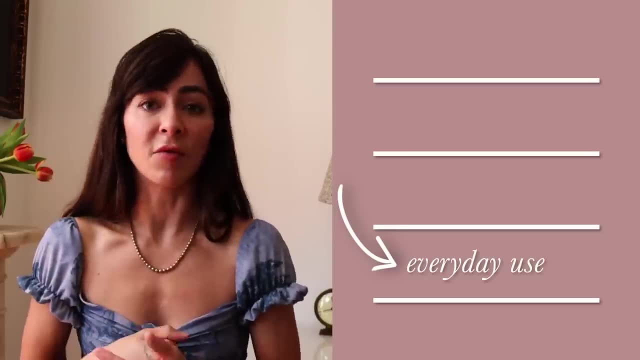 In your bathroom. let's say you got a bunch of shelves- That first shelf that you can easily reach without standing on your toes or pushing up on the counter or moving much stuff, that's got to be your everyday use item, That lotion that you use every day. 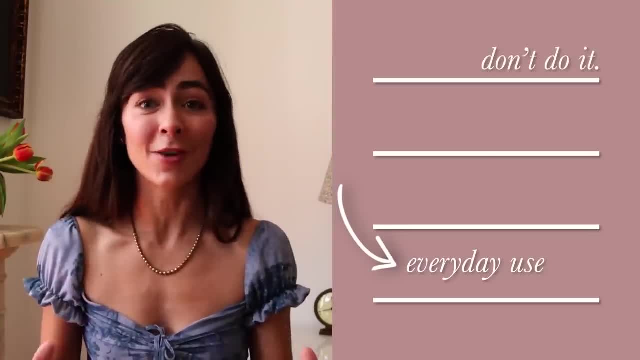 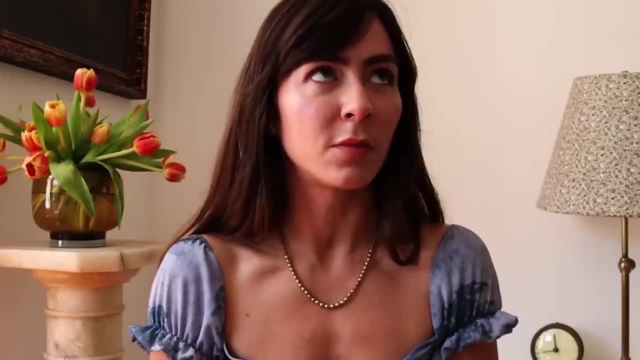 don't make yourself stand on your tiptoes to get it. If possible, don't make yourself do that. When you're doing that every day, you're going to be just a little bit annoyed and it's going to impede and slow down your Wait. I was going to say breakfast routine. That's not the word. 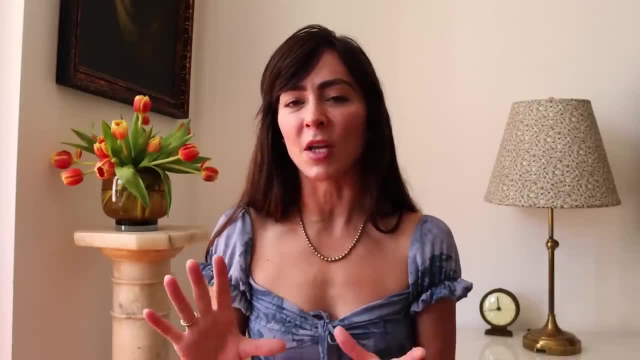 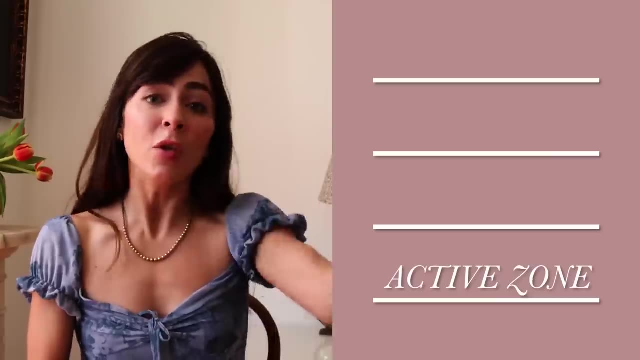 Your morning routine just a little bit more Every time that you do that. all those little speed bumps we got to create flow. so the everyday items- boom, boom, boom. we can reach them. Not only is it easy to get that lotion down that you're going to use first thing every morning. 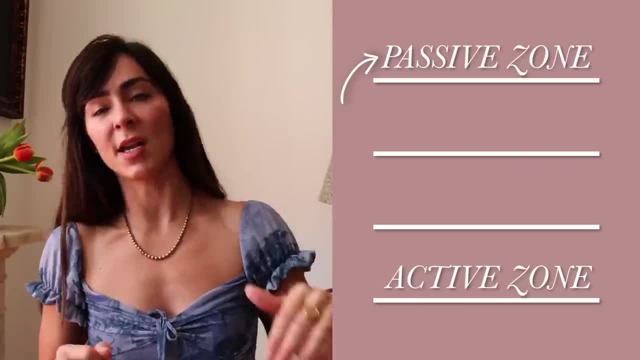 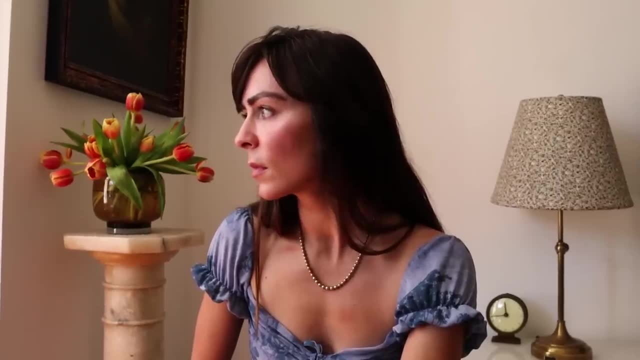 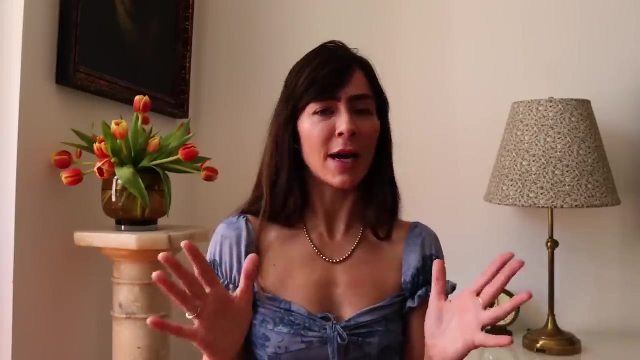 but it's easier to put away. If it's on that top shelf and you have to get up on your toes to put it away, guess what? It's probably going to stay on the bathroom sink most days In your kitchen. If you're crammed for space, don't be putting your melon baller. 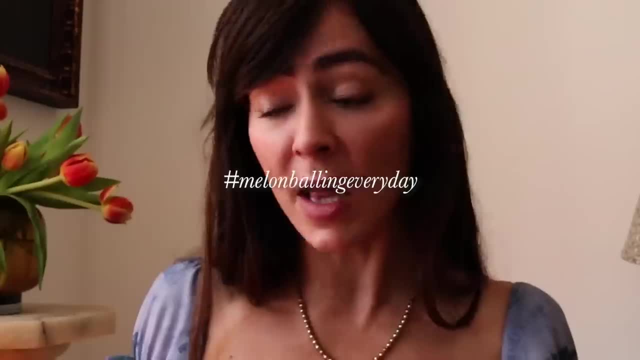 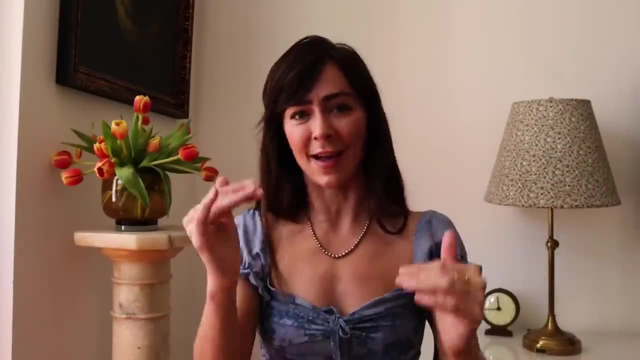 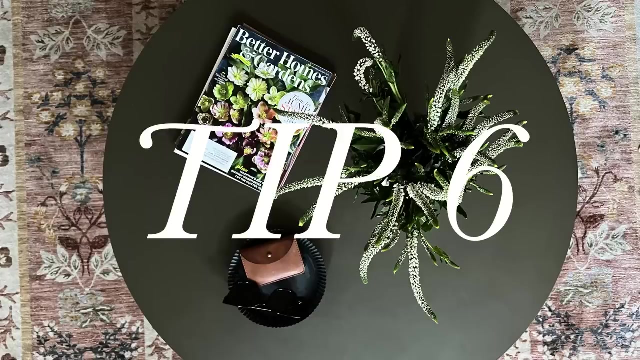 in the forefront drawer or cabinet, Unless you're melon balling every day. get it out of here, put it away. We can use that space for something else. It's prioritizing Ease of access to find your zones. Maximize your weirdness. 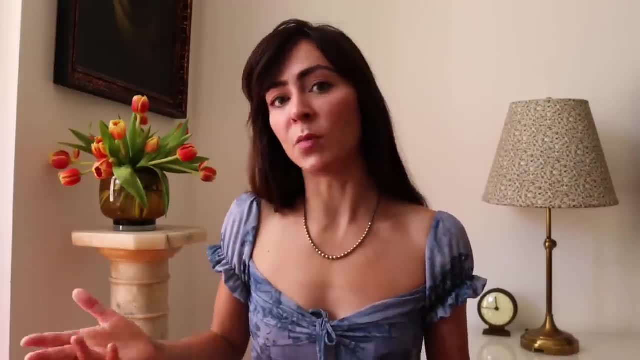 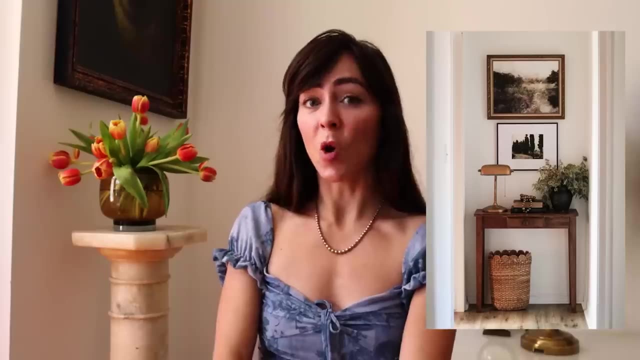 Weirdo spaces. If you're living in, especially a small apartment, like I am, and you're looking at some weird little corner, alcove, and you're like that's a weird space, Guess what That space is going to be, for one of two things You're. 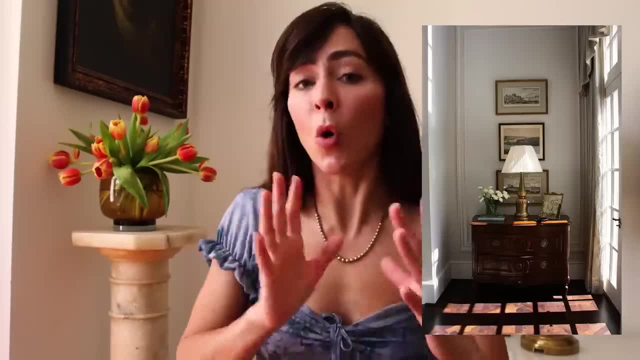 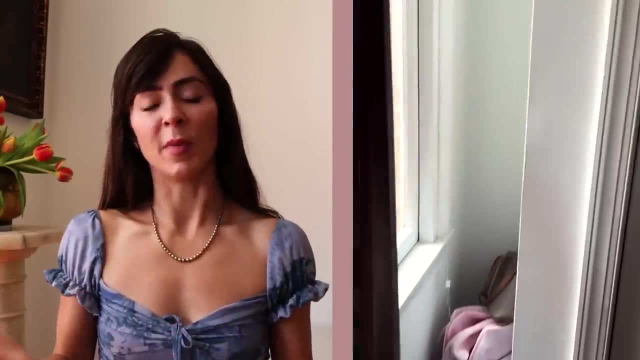 either going to make it into a cute little designed vignette or it's going to be storage And to capitalize on your weirdo spaces. you are going to want a couple great organization gadgets. For example, in my own apartment, in my bedroom, there is this bizarre 10 inches of space. 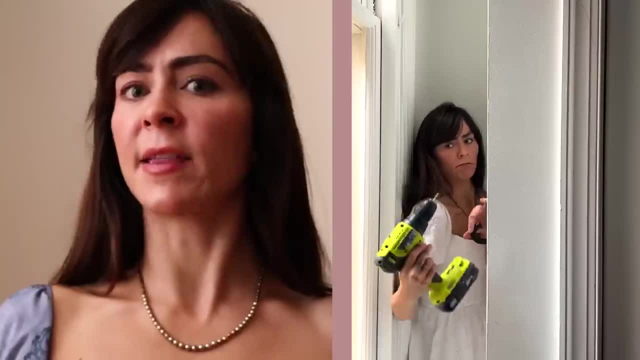 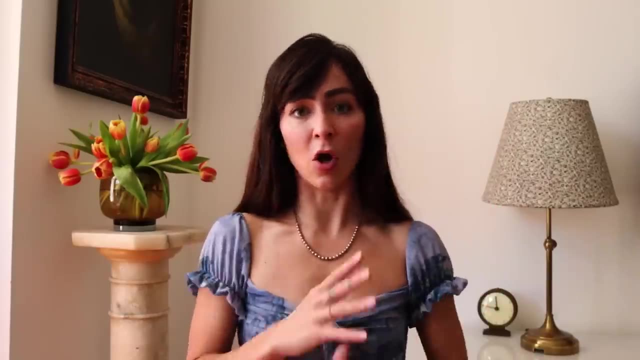 to the side. I'm going to put this in my closet. It feels like that could have been more closet space, but okay, I decided that space is going to hang my purses. It's going to hang my backpacks and all the bags. 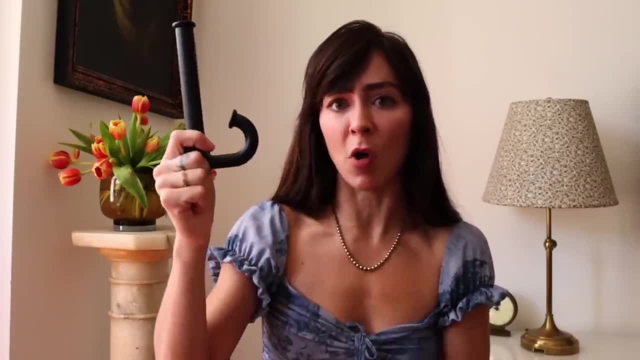 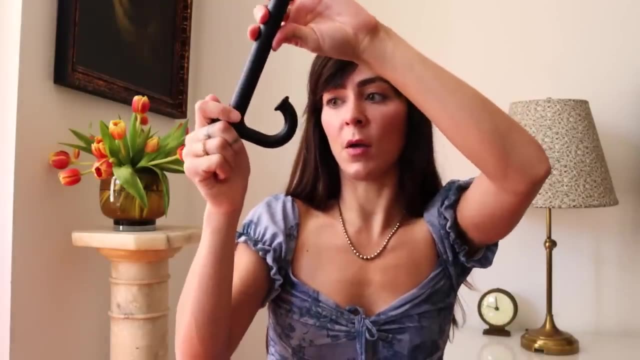 I have. This is one of my favorite tools you can buy. It's pretty heavy duty, It's like very nice quality. I got mine offline. You can get a Chrome version. You can get a white version. Not only is the wall hook, they can go into your wall, but you can lift it up and out to tilt it this way. 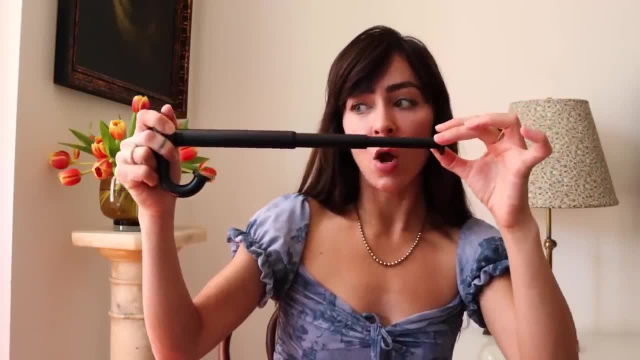 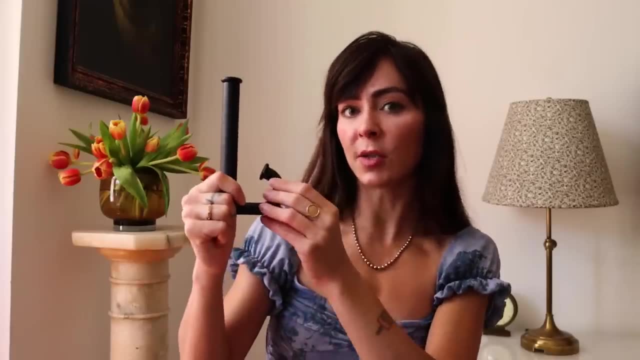 and extend out this way. These are actually intended to go in your closet like a little extend, a hook I think they're called, I don't know. You can put this in your closet to hold belts, to hold purses, and then you can extend it out in your packing, or you're trying to look. 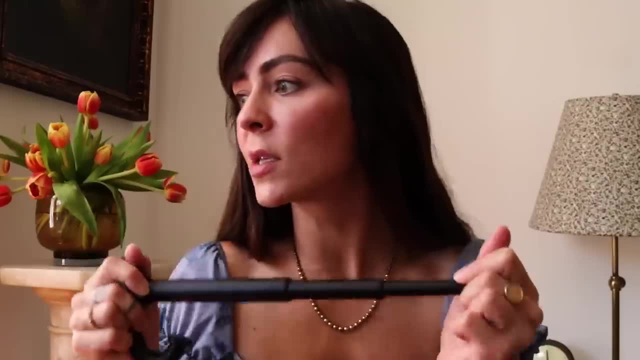 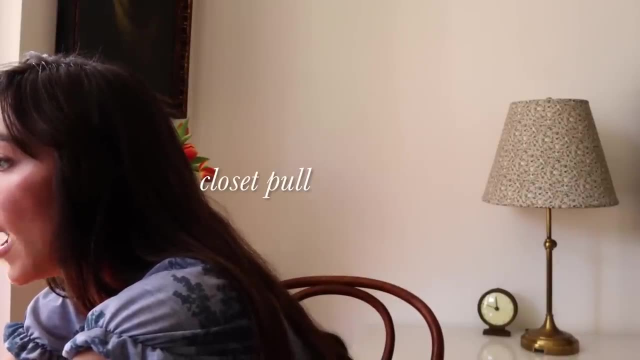 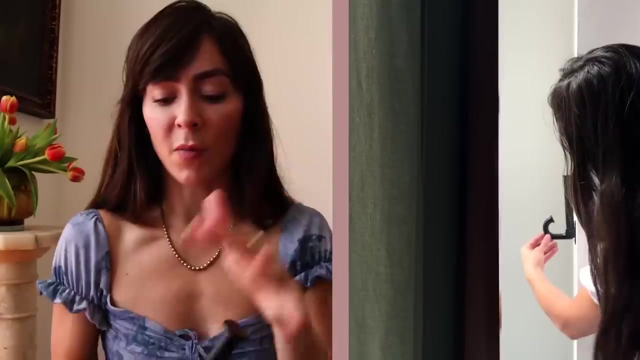 through a bunch of items, hang a bunch of hangers here. It's very helpful. What is the word? What is the word Closet, pull out rod, A valet rod? It's called a valet rod When people do really fancy. 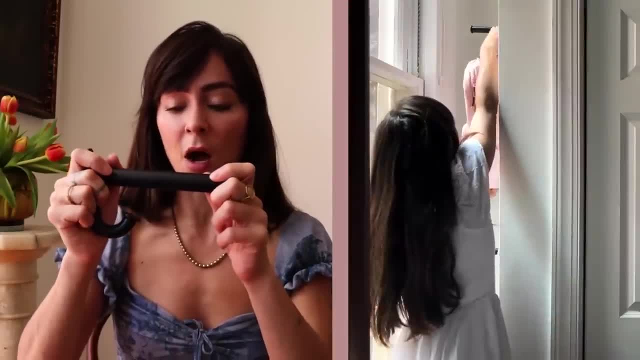 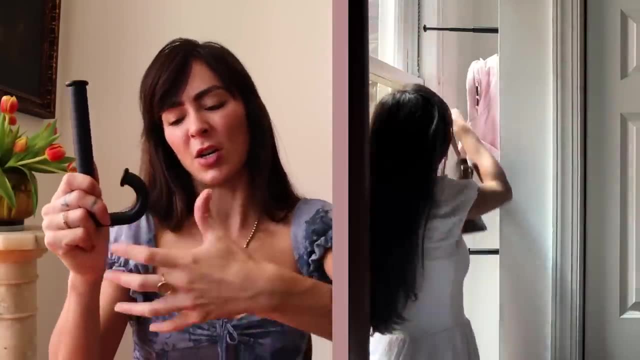 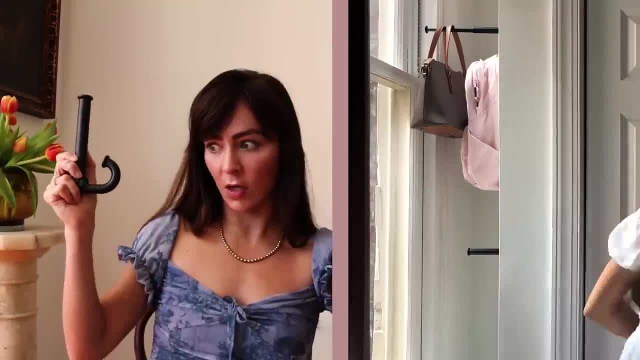 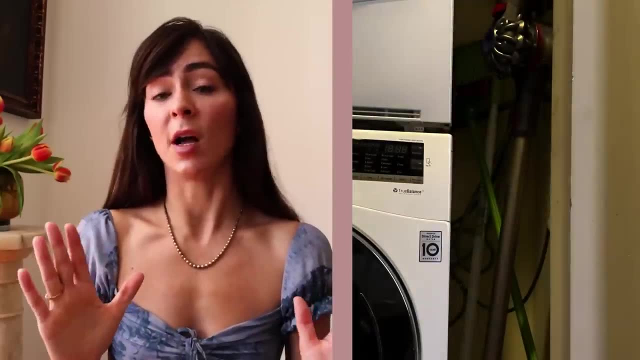 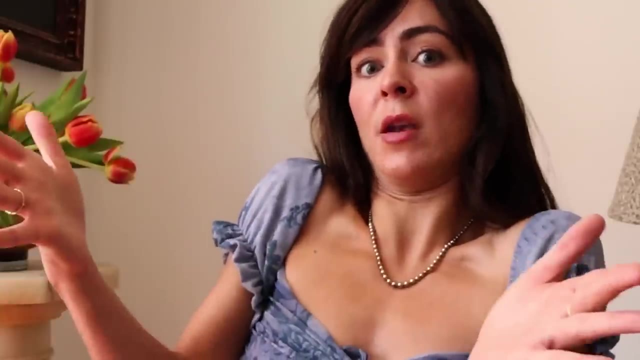 Anyway, love this product. I'm linking everything in the video description. Another weirdo space in my apartment is my little laundry closet. It's also the only closet space in my entire apartment. It's the only storage closet, so I need to make the most of it. There's about a one foot. 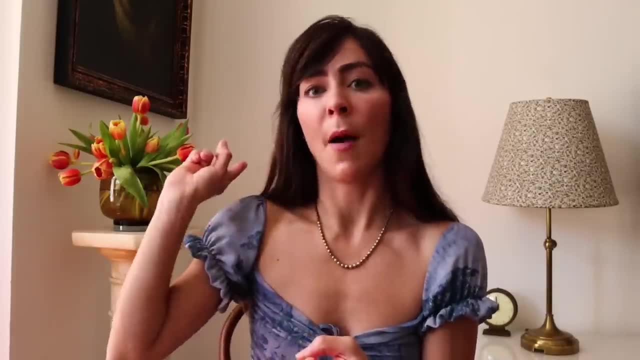 eight inches of space in my closet. There's about a one foot eight inches of space in my closet. There's about a one foot eight inches of space in my closet. That's where I'm putting my broom, my vacuum, my what's it called Dustpan. That space is going to be chock full of these little. 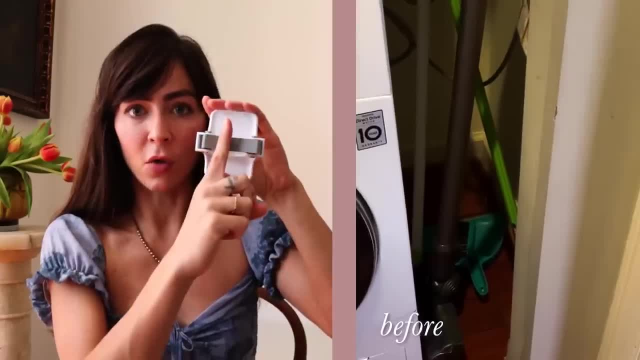 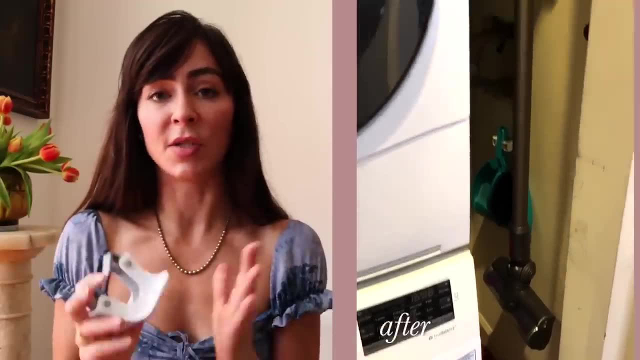 dingle dangles, It attaches to the wall with a command strip and then you can hold your broom, just like that. It clamps it. Everything is being held up. It's getting up and off the floor in those tight little spaces. It's made it so much tidier, so much easier to access stuff. 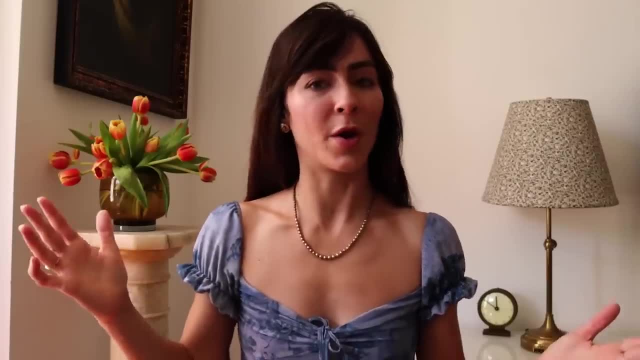 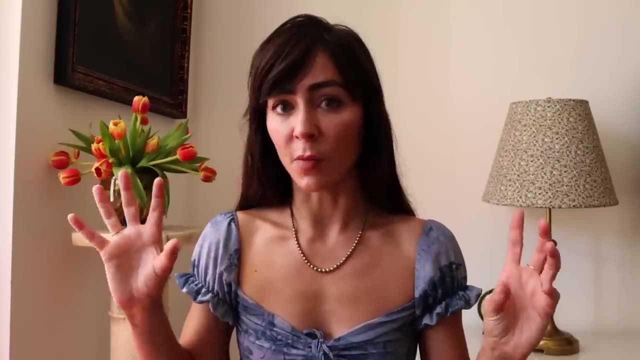 These are a must for me. Another weirdo space under your sink. What a weird chaos of a world that always is It's organization. hell, Maximize that weirdo space. There are some great products. I like to do just an over-the-cabinet door. 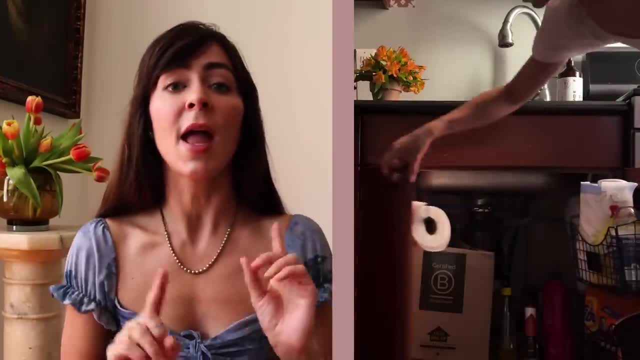 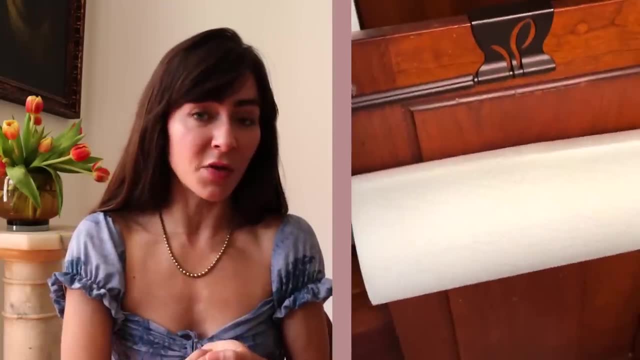 I found this specific combination of this paper towel holder and this over-the-door rack that can stack together. I have them on two separate doors. You can put your paper towels on this holder, but you can also put a roll of your trash bags. put all your storage stuff in the door. 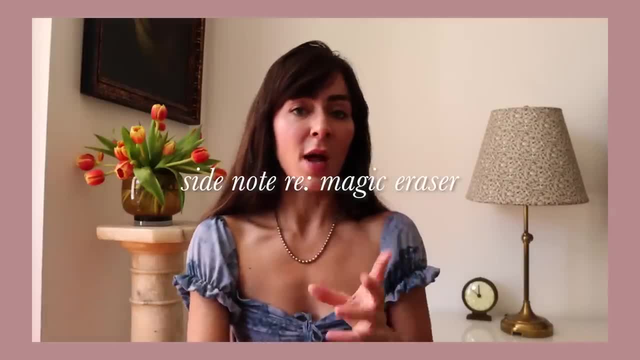 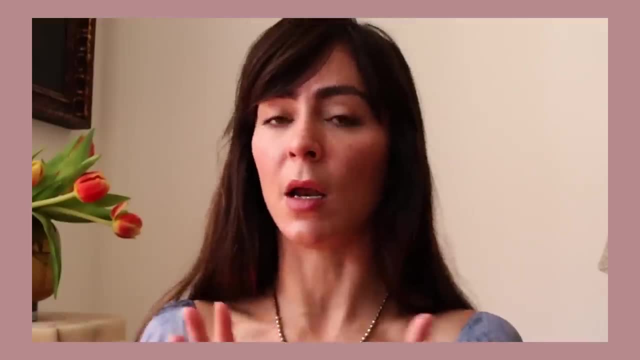 Maximize that space. These ones very worth it. Side note, I also keep my magic eraser in there, The magic eraser. if there's nothing else, you buy the magic eraser. I mean I don't want to over-hype the magic eraser. 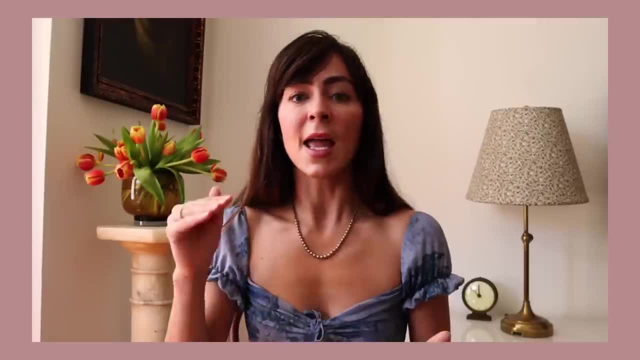 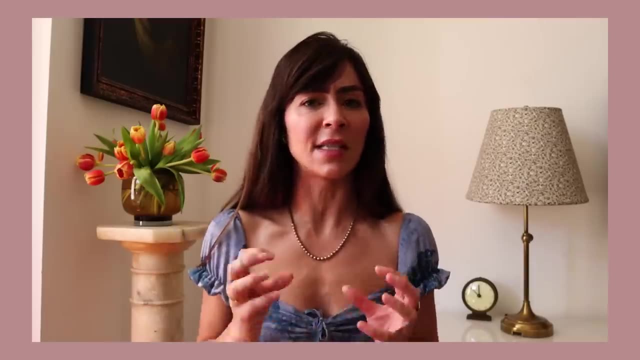 but there's nothing else that I believe in as much as this product. It gets all of those fingerprints off your wall, all those scuff marks. I clean my white sneakers with them. I have removed stains from marble. This is not sponsored, I can't tell you. 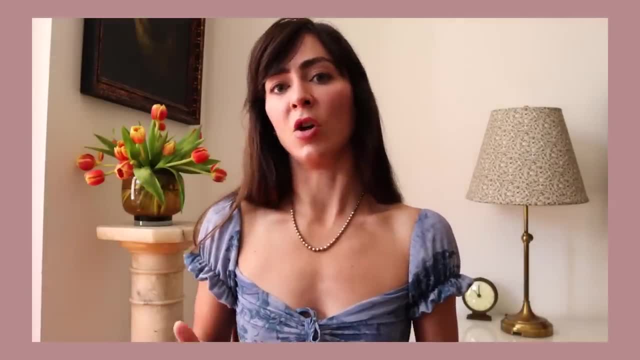 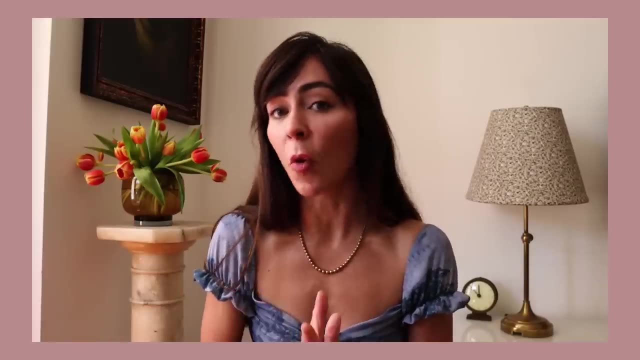 I hope the guy who invented this, the magic eraser, is living a good life. I wish him all the happiness in the world For the way that he has changed my life. If I have something that is scuffed up before I get rid of it, try the magic eraser on it. I don't care what the damage is. 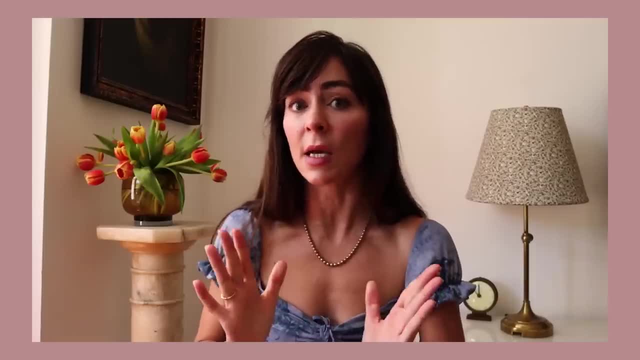 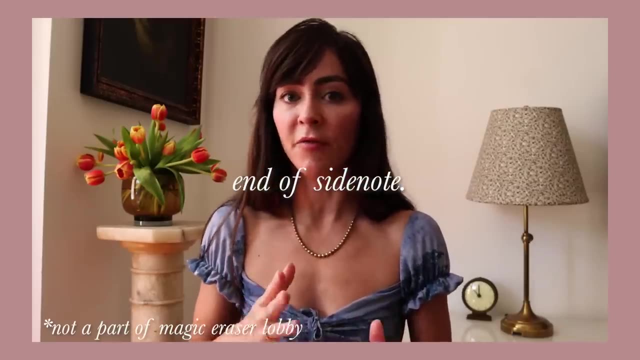 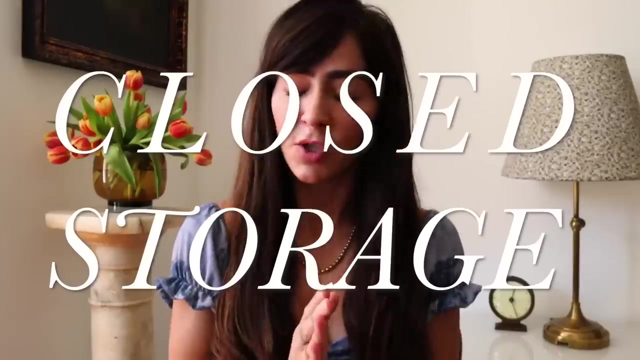 it probably helps. It's amazing. It's amazing. Okay, The end, That's the end. I'm not. I have no association with the magic eraser lobby. I'm just a very big fan. Closed storage, Closed storage. This is so important when you're buying a piece of furniture. 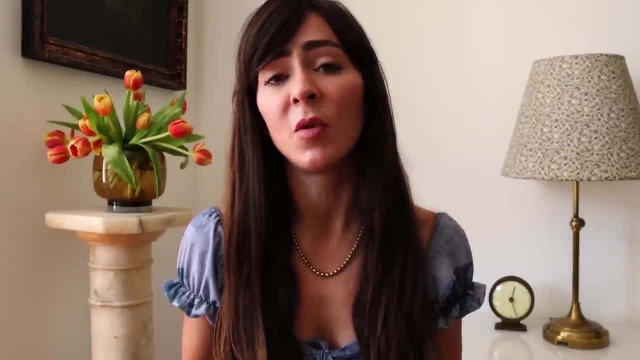 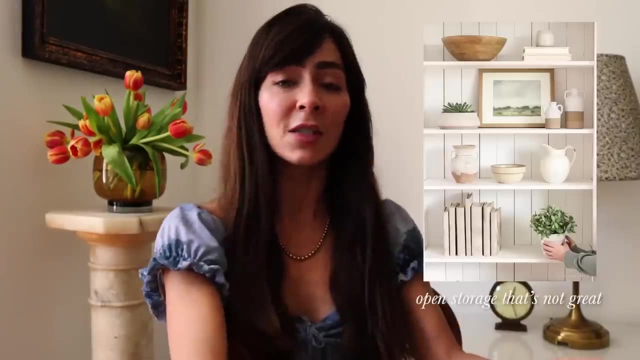 you're buying storage items for yourself. Just give your self a break. You make your life a little bit easier. I usually opt for the closed storage. Now there's some open shelving. It's really beautiful and nice and it looks great on the. 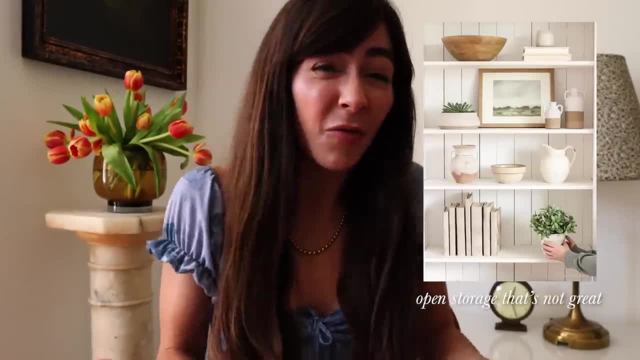 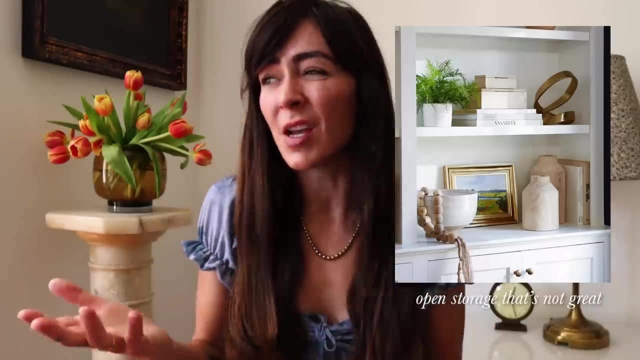 Instagram photo. but it's not usually actually great for storing stuff. We end up putting like the wooden beads on there, or we buy a vase just to go on the shelf because there's nothing we already own that we would be visually happy with storing on the shelves. I don't know. 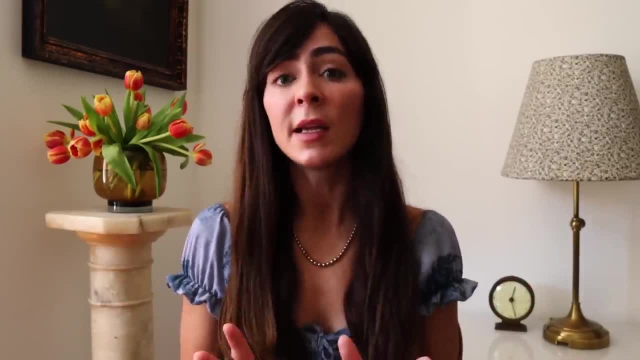 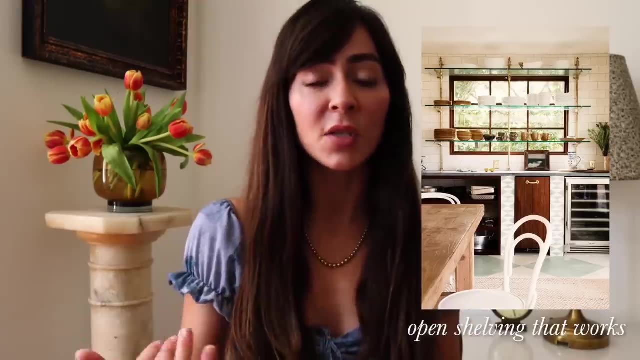 It's a weird thing. That being said, open shelving can be really nice sometimes in your kitchen to give up too much cabinetry, to give the eye a break, Usually if you have open storage, open shelving and you're really using it to store a lot of stuff. if I can, if I can afford to go the 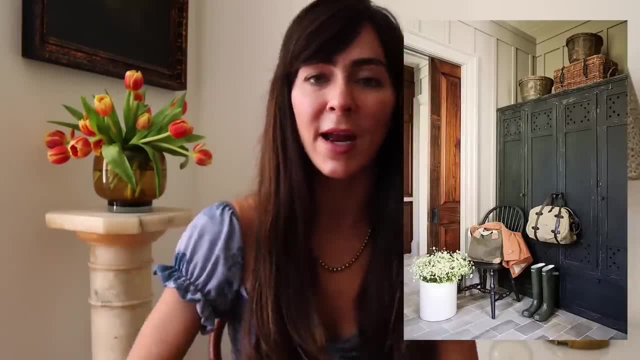 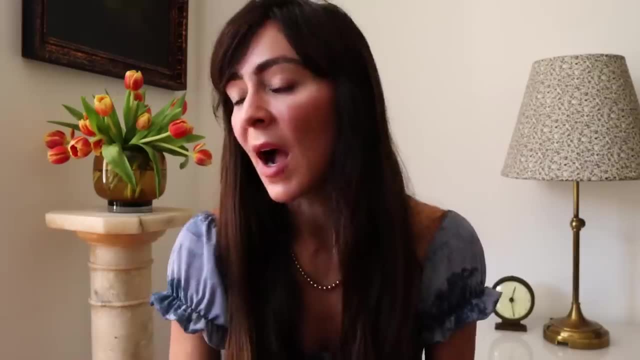 closed storage route. I do the closed storage. Give yourself a break. put your batteries and your electronics and all that stuff in organized baskets, Then close the door so you don't have to think about it. I think that the open shelving is great for storing things that are easy to look. pretty, your glassware, your dishes, your books. But if you're going to store all of your furniture, you just need to be very, very careful about it. If you're like, I'm not going to open up this one. 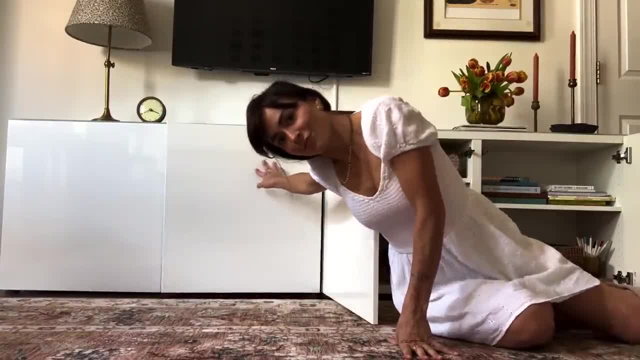 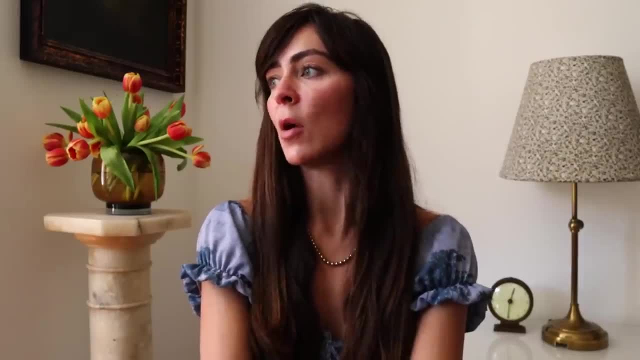 but if you're getting a credenza, you're getting a sideboard or something. i would just go the closed storage route as much as you can, just give yourself a break. yeah, you know, i don't have time to make home organization my entire identity. i don't have time to make storage containers. 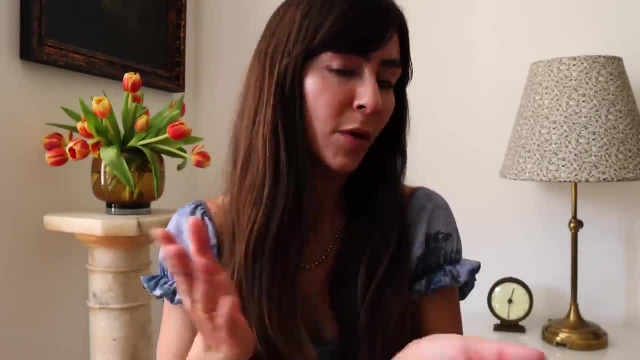 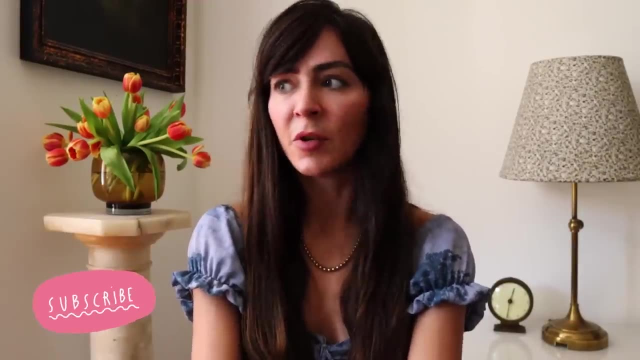 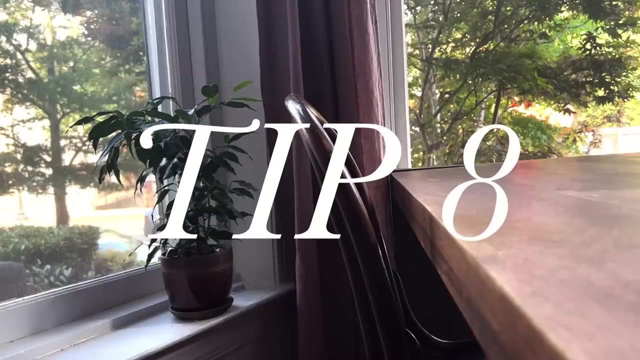 my whole personality. so if you feel the same way, remember to like the video. subscribe for more stuff like this. it's a good time on here. i'm all about making organization or design accessible and realistic to real people living real chaotic lives. all right, tip number eight: you want to subdivide? this is especially important for junk drawers, where 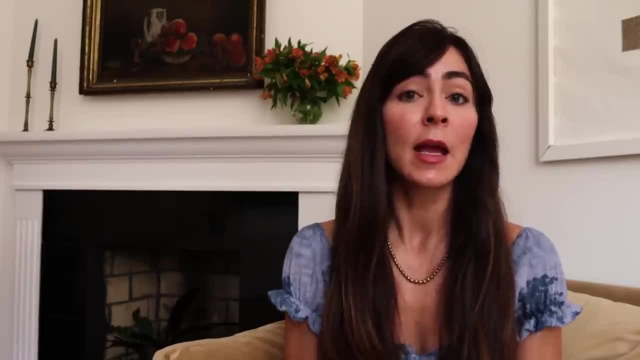 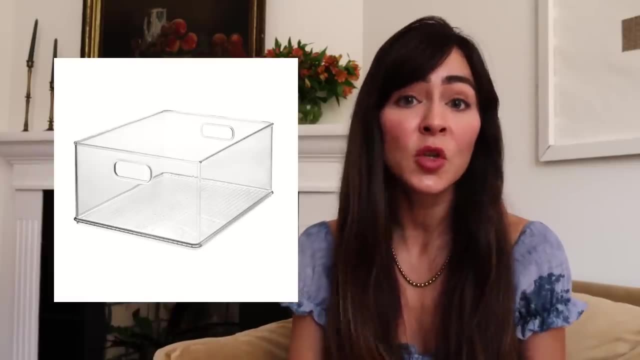 there's just like a ton of stuff being held and i will say the organization product you probably don't need to invest in is a million of those clear containers from the container store. they're nice but, dude, they're super expensive, even getting a bunch of them from goodwill or a bargain store. 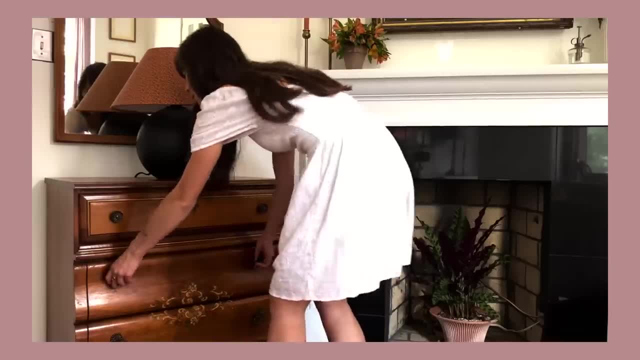 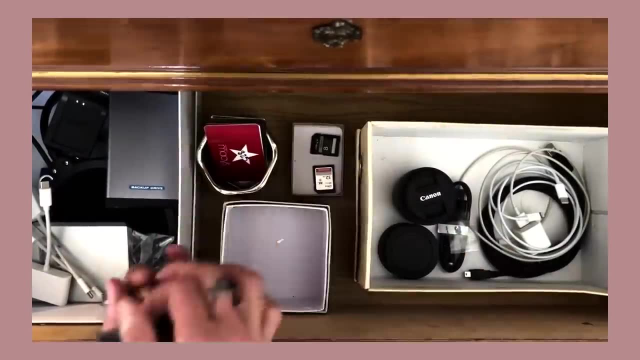 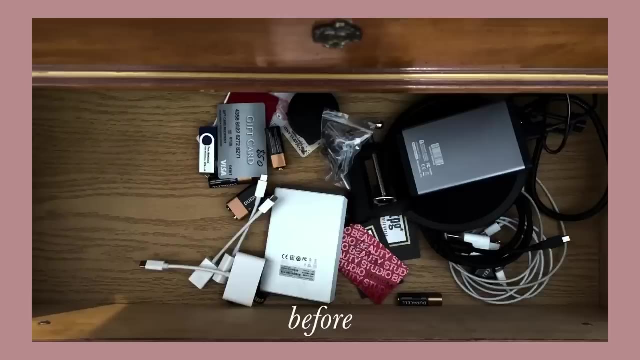 like it's a lot of stuff and it's not necessary. in my home i'm using shoe boxes, gift boxes, to organize and compartmentalize. you can do the fancy containers. you can also get um like the drawer expanders. whichever way you want to do it, you do want to subdivide. it will make a world of difference, especially in those really. 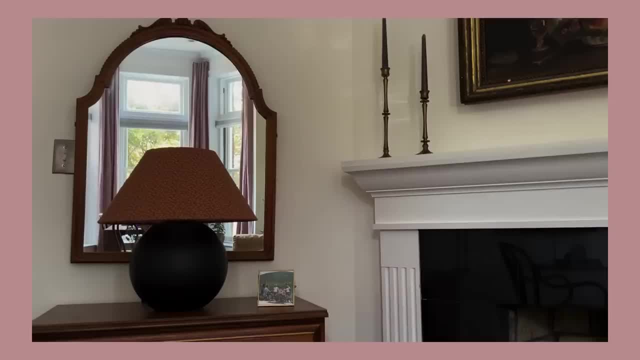 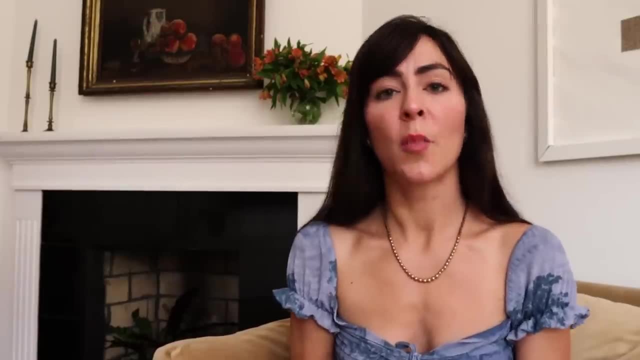 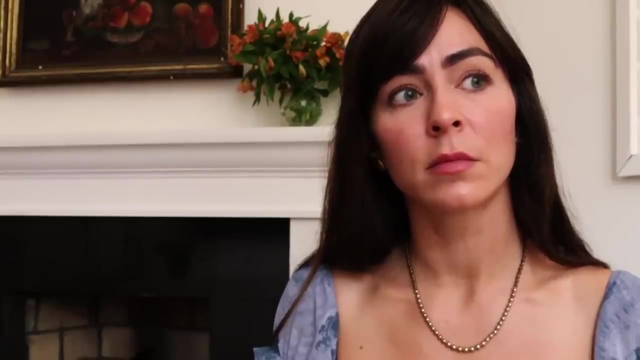 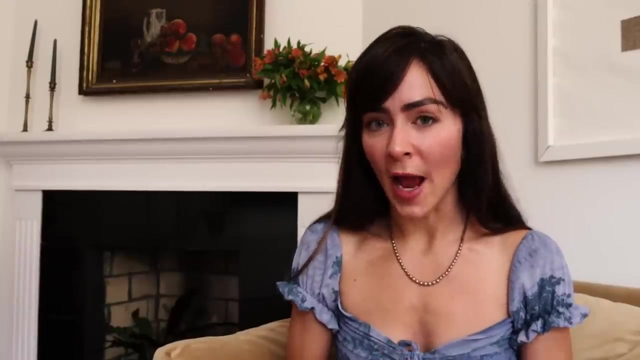 cluttered storage areas where you got to keep a ton of stuff. tip number nine is probably the most important one: purge, purge your stuff, declutter. it doesn't matter how much you organize if at the end of the motorcycle okay, thank you. it doesn't matter how much you organize if you just have too much stuff. 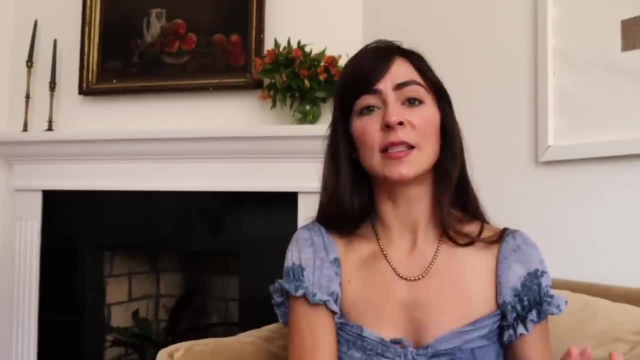 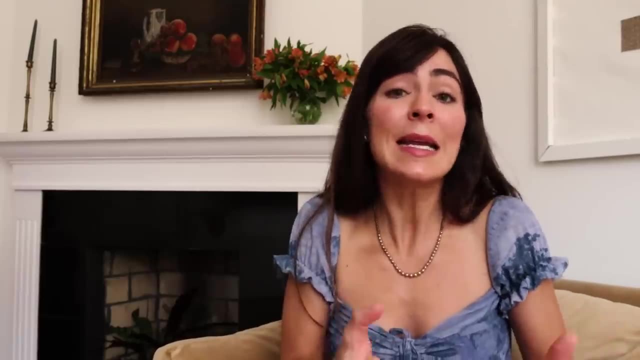 and if you're anything like me, you do most likely the things that are over cluttering your home you don't need. purging your home is not just something you need to do once a spring. it needs to be an easy light lift that you can do a little bit every week, every month. here's some easy. 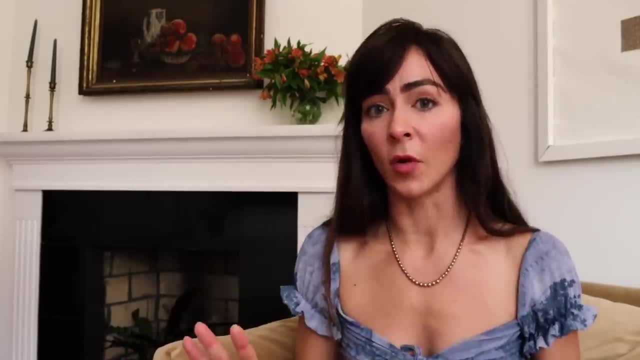 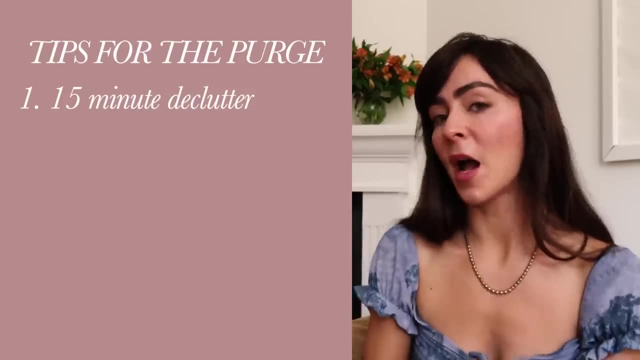 tips to help accomplish a declutter, a purge, that's not going to overwhelm you. declutter for 15 minutes. set a timer and do what you can do in 15 minutes. put stuff in the donation pile, in the throwaway pile. 15 minutes, that's all you got to do. i heard this from another organization. youtuber- do it on. 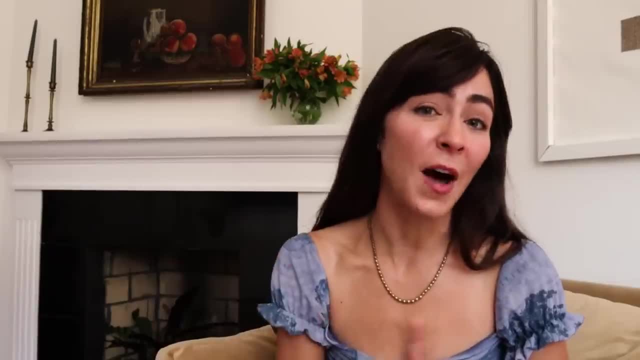 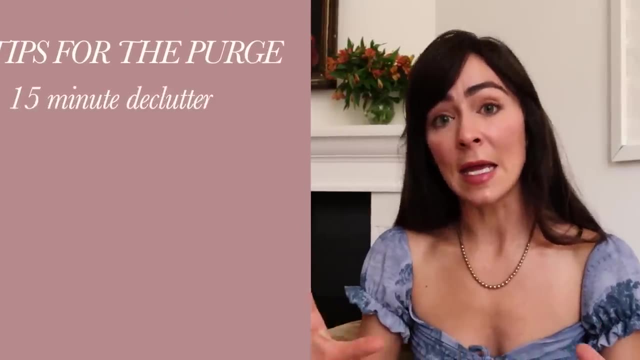 a dime. check out her stuff. she's wonderful. if it takes me more than five minutes to tidy up any room, i need to start getting rid of some stuff. five minutes, it shouldn't take more than that. if it's taking you more than that, you got to get rid of some stuff in that house. another tip set a. 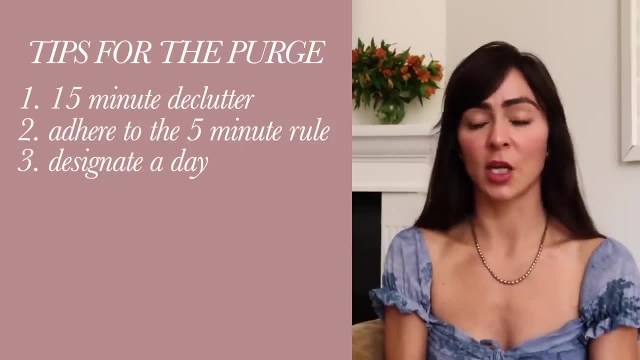 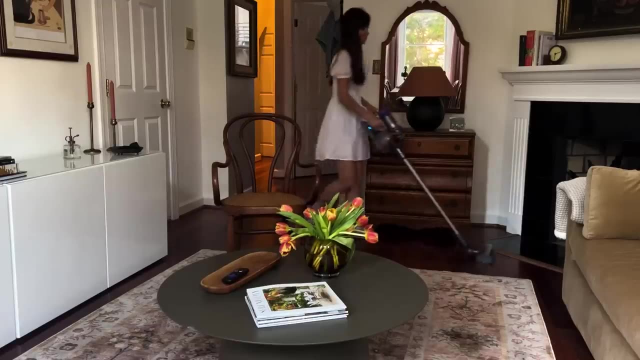 your day of the week where you're doing that intentional home organization on sundays. sundays are the day i take out the trash, i vacuum, i sweep, i pick one thing to try and organize or declutter. just have it built into your schedule. you can have your kids, kids freaking like cleaning stuff. i don't. 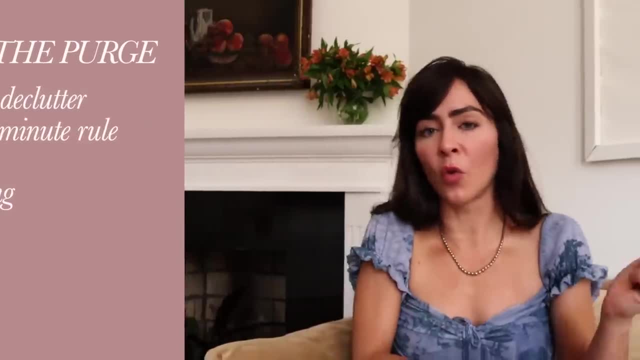 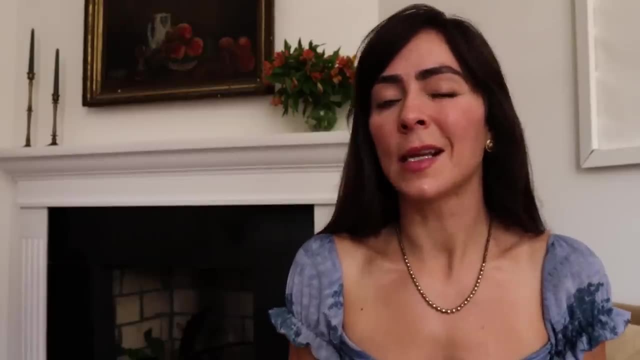 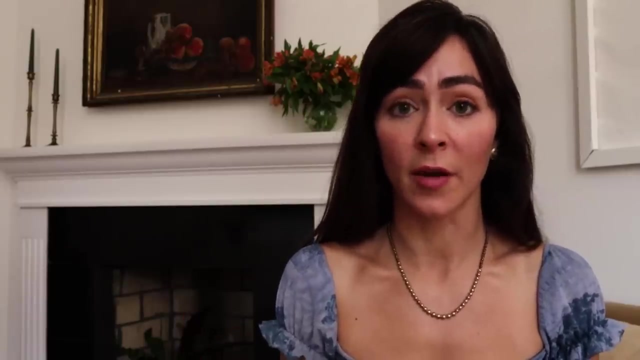 know what's wrong with them. you give them a spray bottle. you give them some fancy gloves, a cool broom. they're into it, okay. so we know what decluttering and purging looks like, but sometimes it's still so hard to do because it's extremely emotional for a lot of us. we have 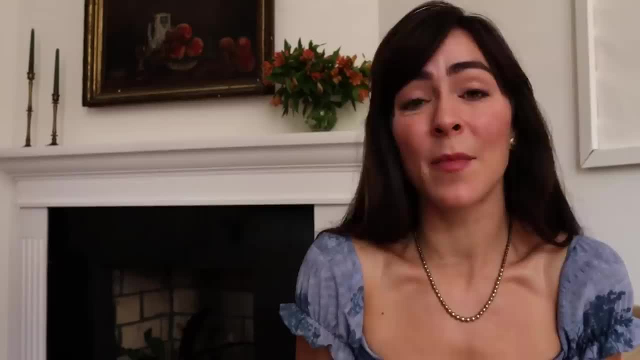 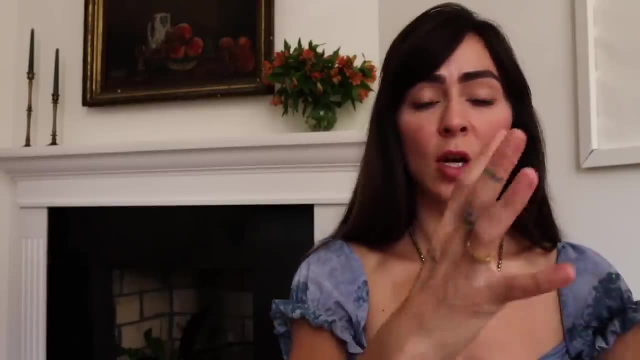 sentimental attachment to items or we just feel obligated to hold on to them or even guilt over letting them go. so here are some tips for managing the emotional endeavor of decluttering. i think marie kondo's you know concept of what sparks joy and what doesn't. you hold on to things that 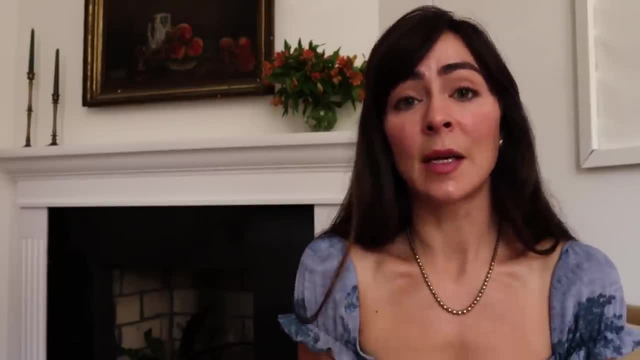 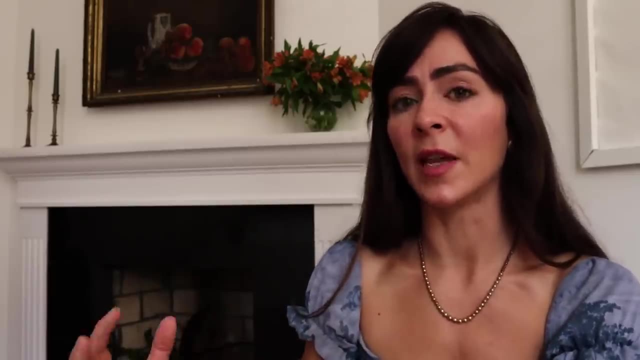 sparks joy, you let go of things that don't. it's super helpful and that's lovely. but sometimes, for me personally, it's hard to distinguish even something that sparks joy, or something that the idea of letting it go just sparks fear and i feel obligated to hold on to it, or i feel guilty if i don't hold. 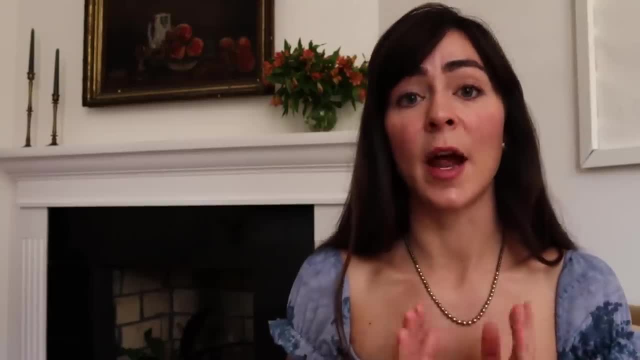 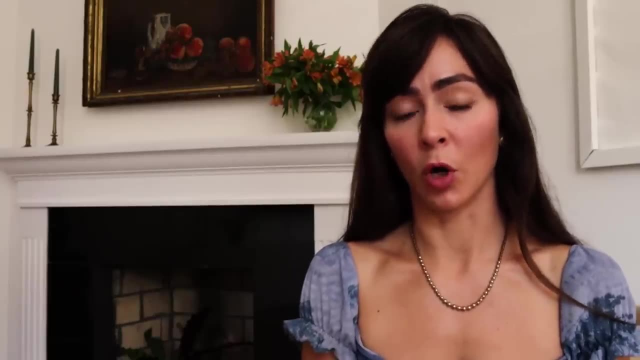 on to it. it's hard to distinguish those things, so here's a different tip that helps me when deciding what to keep and what to get rid of. if this item was covered in red wine, how hard would i work to save it? how hard would i work to revive it? if it's something that you're like, oh man, if that got. 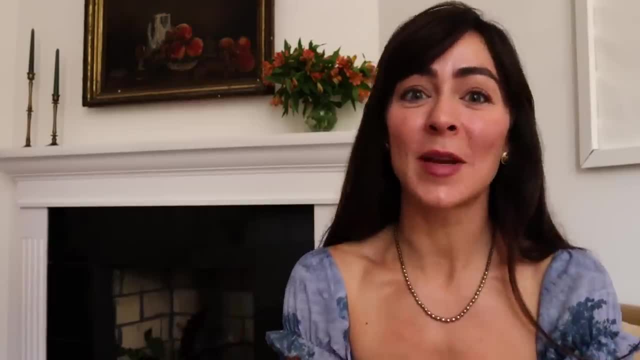 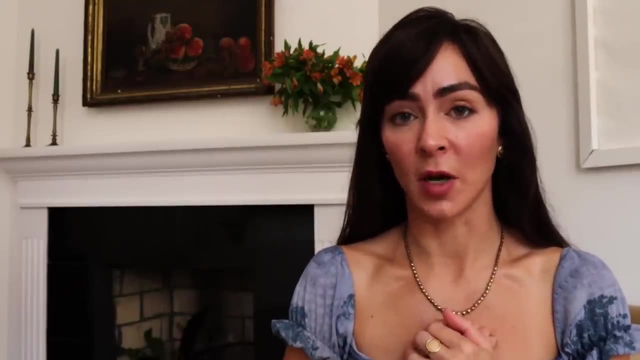 covered in red wine, i would be so relieved to be able to say: yeah, it got ruined, sorry, i couldn't hold on to it. that helps me to really distinguish what i'm doing and what i'm not doing, and i can't distinguish what items i'm only holding on to for obligation. it's easier said than done, but let go. 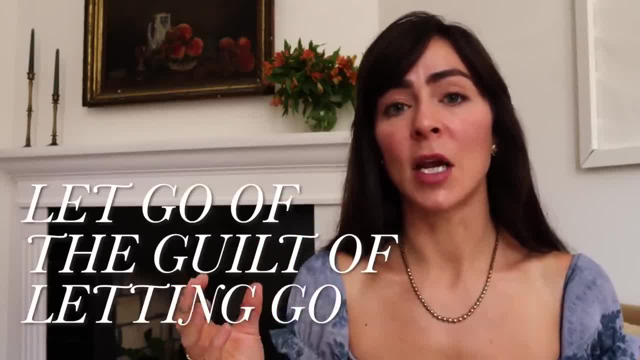 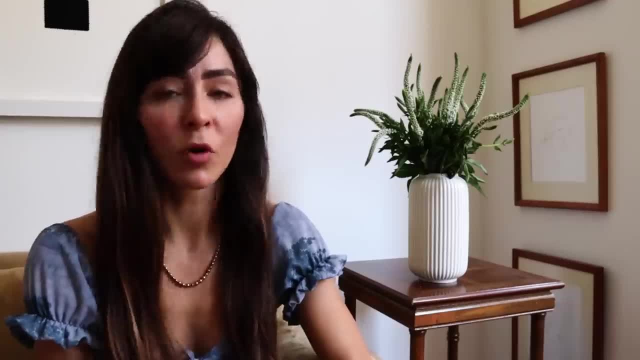 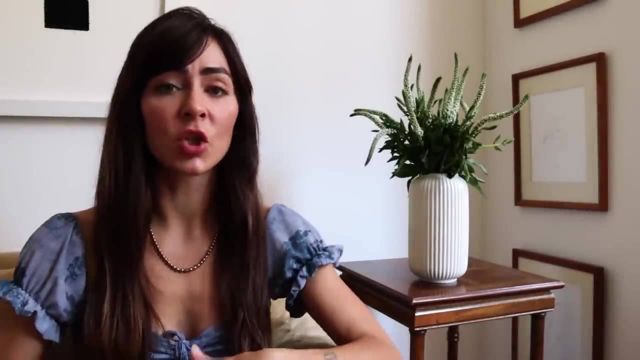 of the guilt of letting go when that idea clicked. it was a huge and life-changing lesson for me. i'm not an organization freak- i haven't made it my whole personality, but it affects interior design, which i love. good organization should let all the beautiful items in your home.